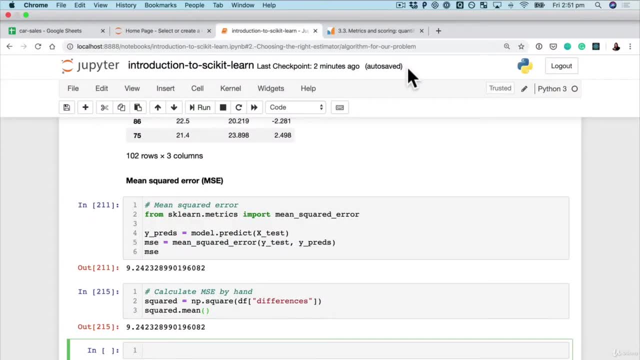 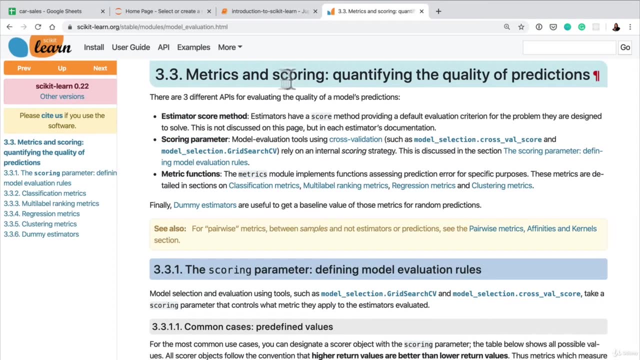 Whoa, we've really covered a bunch, but we haven't even touched the scoring parameter. And, as a refresh, the scoring parameter is one of the second ways that we can evaluate a model right, So the scoring parameter is used with model evaluation tools that use cross-validation. 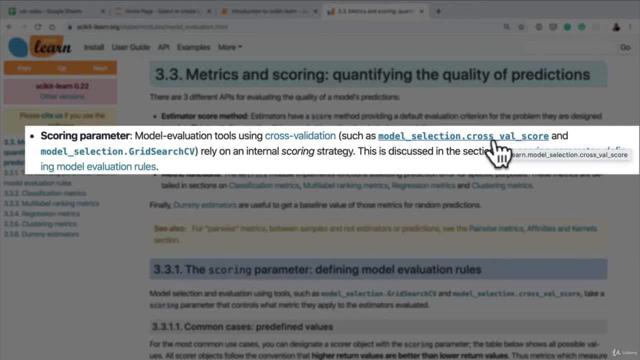 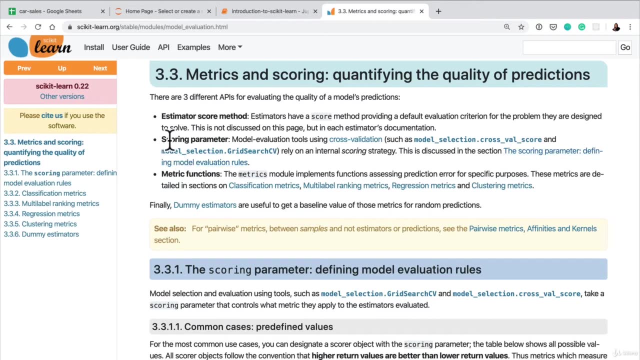 such as modelSelectioncrossValScore- We've seen that one before- And modelSelectiongridSearchCV. Now, we haven't seen that one before, but what we're going to do is check out how we can use the scoring parameter with cross-valScore. Before we do so, let's set up a little heading. 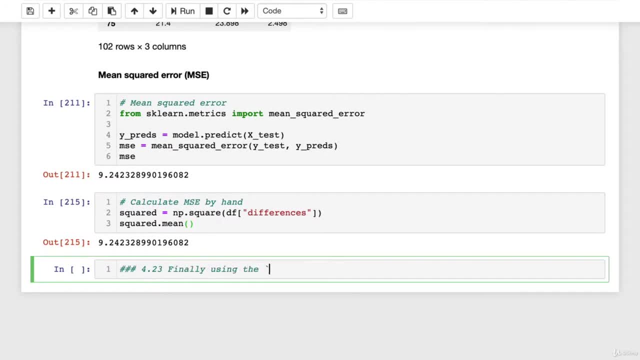 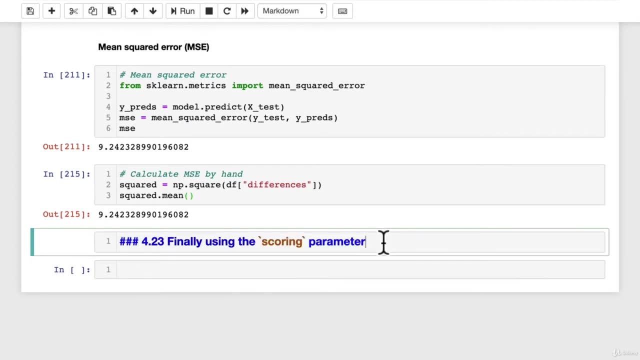 Let's remind ourselves, finally, using the scoring parameter- And I know there's a lot to take in right, And I don't expect you to know everything like straight away- It's going to take a little bit of practice, a little bit of time, a little bit of effort for these things to start to sink. 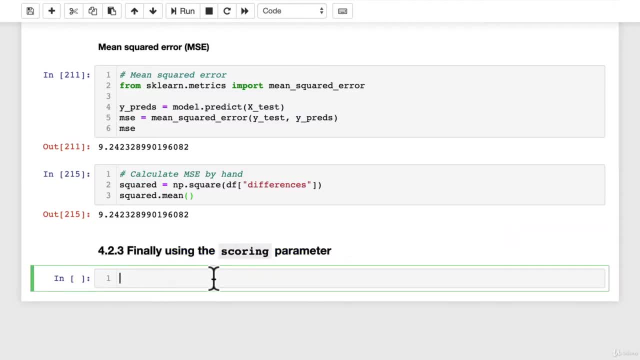 in right. So here we go, finally, using the scoring parameter. And speaking of practice, it's one of the reasons why we keep practicing writing out, building machine learning models and splitting our data. So for model selection, we're going to. 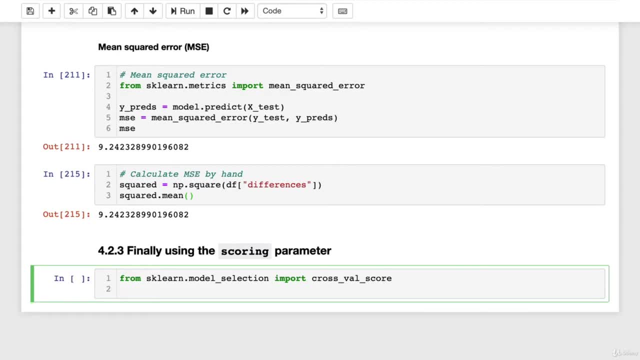 import cross-valScore, because that's where we can use the scoring parameter. And then we're going to import our random forest classifier. Import random forest classifier- Yep. And then we can go nprandomSeed 42, our favorite number. Again, you could use almost any number here. I. 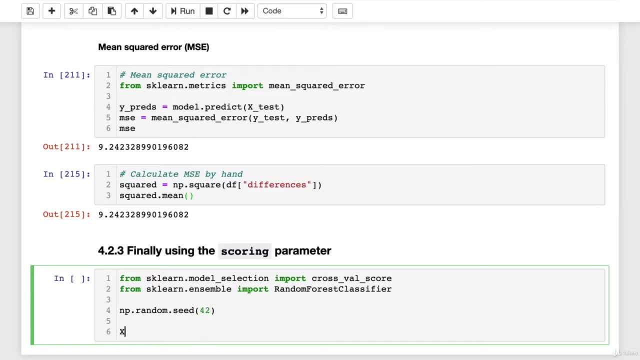 actually really like the number 72, but 42 will do. X equals. we'll set up our X data. heart disease dot drop Target axis equals one beautiful Y equals heart disease Target. there we go, And now we can set up a classifier And we're going to. 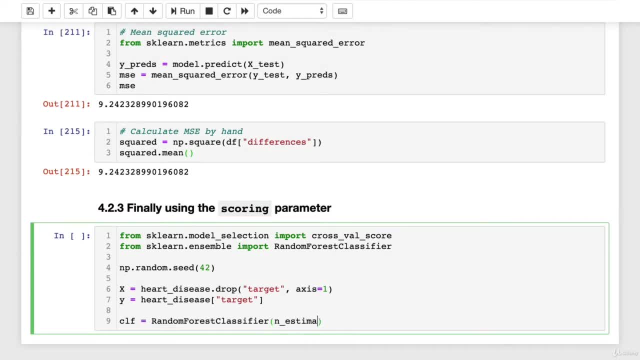 use, of course, random forest classifier, our favorite, the warhorse of machine learning. We'll set number of estimators to be in 100, so we don't get that pesky little warning that we've been getting. And we're going to set number of estimators to be in 100, so we don't get that. 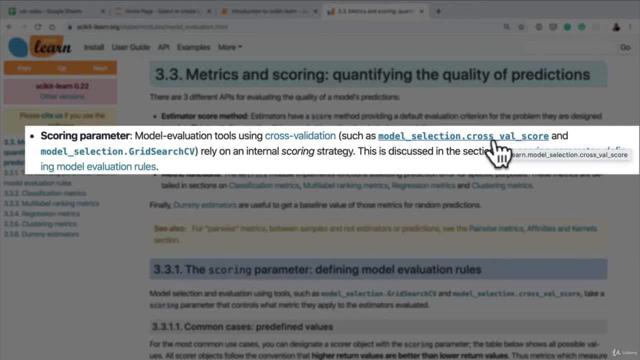 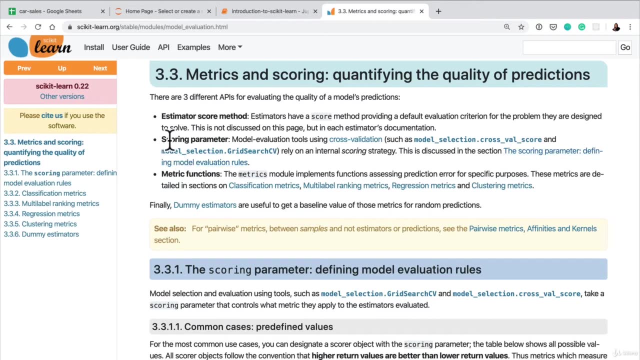 such as modelSelectioncrossValScore- We've seen that one before- And modelSelectiongridSearchCV. Now, we haven't seen that one before, but what we're going to do is check out how we can use the scoring parameter with cross-valScore. Before we do so, let's set up a little heading. 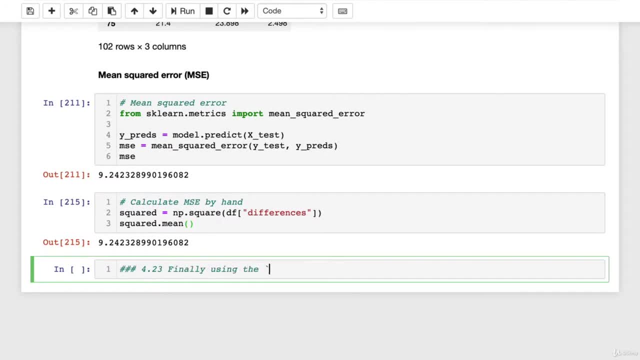 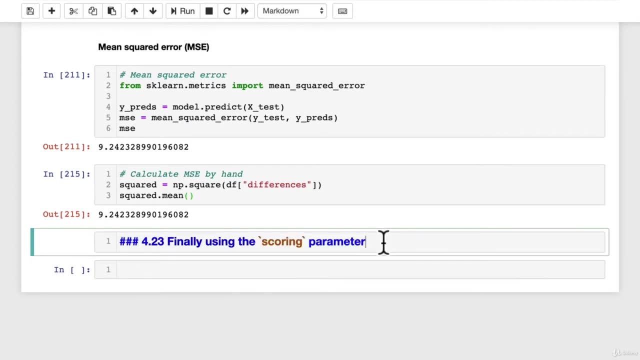 Let's remind ourselves, finally, using the scoring parameter- And I know there's a lot to take in right, And I don't expect you to know everything like straight away- It's going to take a little bit of practice, a little bit of time, a little bit of effort for these things to start to sink. 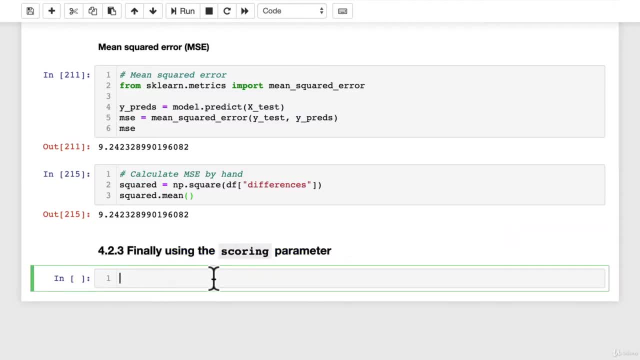 in right. So here we go, finally, using the scoring parameter. And speaking of practice, it's one of the reasons why we keep practicing writing out, building machine learning models and splitting our data. So for model selection, we're going to. 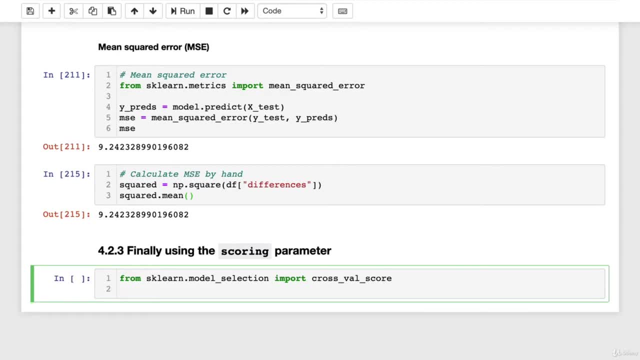 import cross-valScore, because that's where we can use the scoring parameter. And then we're going to import our random forest classifier. Import random forest classifier- Yep. And then we can go nprandomSeed 42, our favorite number. Again, you could use almost any number here. I. 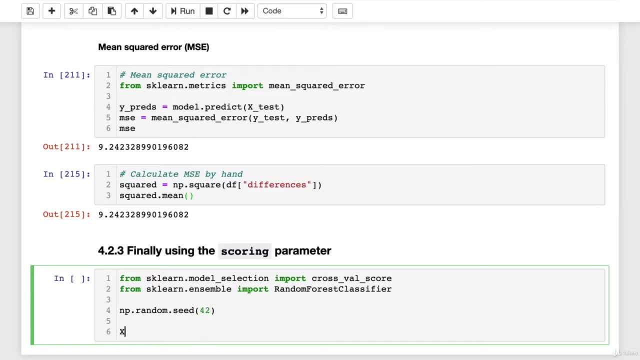 actually really like the number 72, but 42 will do. X equals. we'll set up our X data. heart disease dot drop Target axis equals one beautiful Y equals heart disease Target. there we go, And now we can set up a classifier And we're going to. 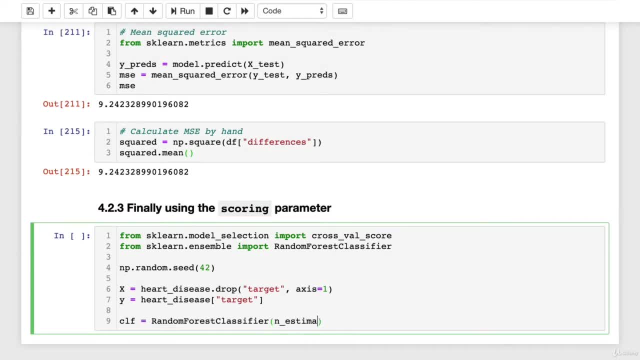 use, of course, random forest classifier, our favorite, the warhorse of machine learning. We'll set number of estimators to be in 100, so we don't get that pesky little warning that we've been getting. And we're going to set number of estimators to be in 100, so we don't get that. 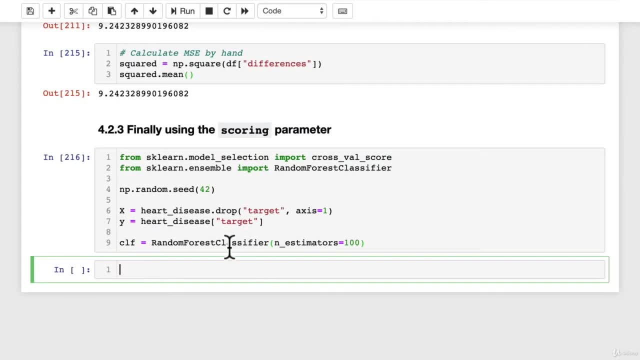 pesky little warning that we've been getting And we'll do that Beautiful. So we've instantiated our machine learning model. It's ready to be fit, So we can do that here, nprandomSeed. We'll do it again And we'll go cvac. Why are we doing cvac? Well, we'll see in a second right. 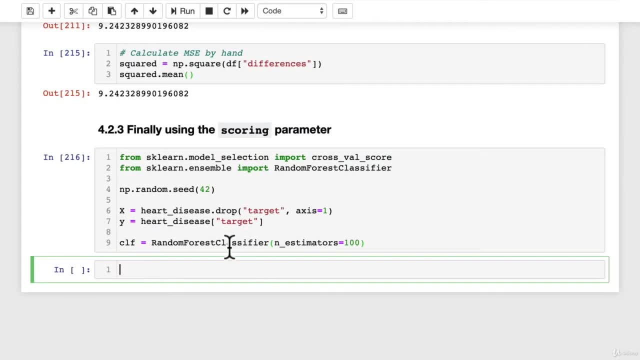 pesky little warning that we've been getting And we'll do that Beautiful. So we've instantiated our machine learning model. It's ready to be fit, So we can do that here, nprandomSeed. We'll do it again And we'll go cvac. Why are we doing cvac? Well, we'll see in a second right. 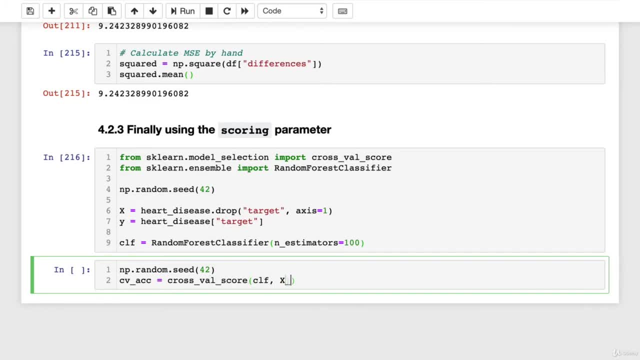 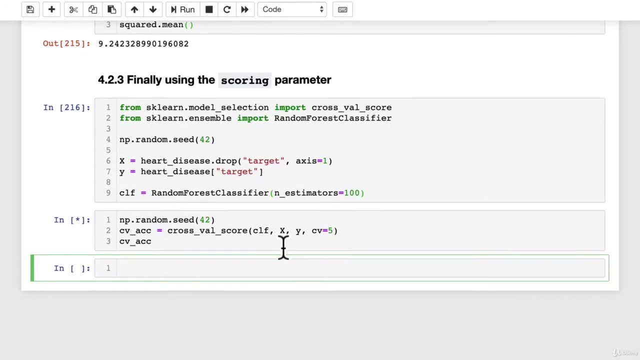 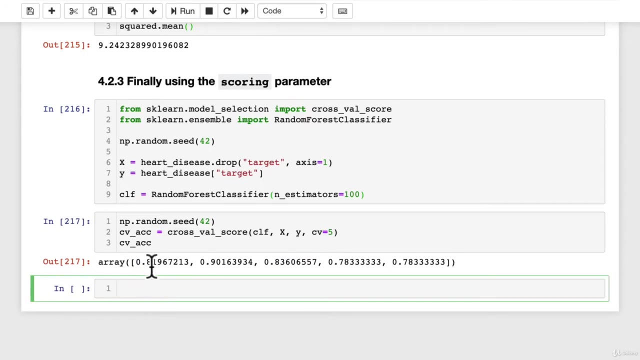 Cross-valScore, clf, x, y, and then we'll use five-fold cross-validation, cvac- Wonderful, It's going to train five models, evaluate them on different test sets, And then, of course, we could take the mean of this. 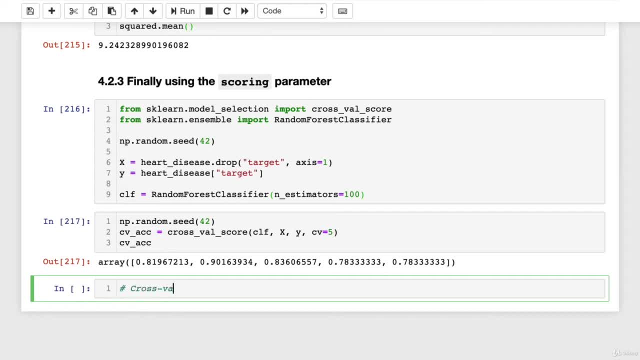 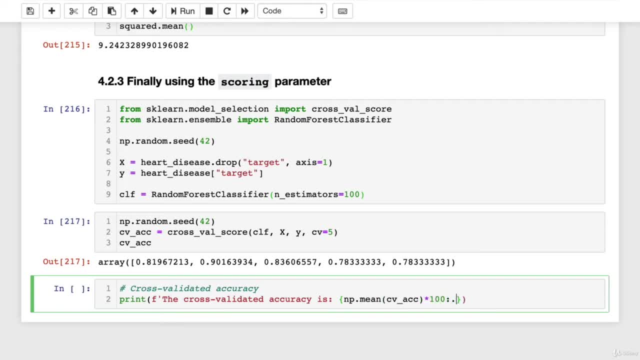 that to. We'll only use cvac, And then we're going to take that to. We'll only use cvac, Times 100 and two decimal places And we'll put a little percentage sign on the end And we need a final string. 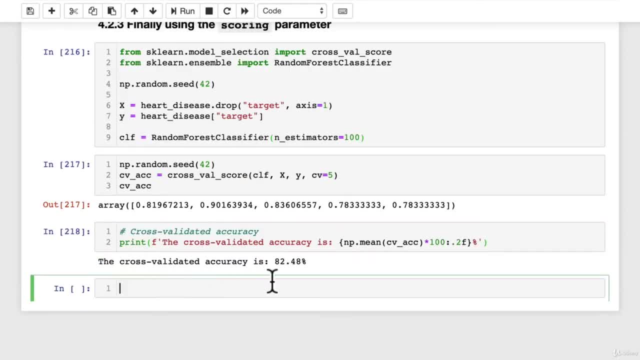 delimiter, Beautiful. So now the cross-validated accuracy is 82.48%. Now, we've seen this before, right, We've seen this line, We've seen this line. And the reason why is we're using this is because, by default, the model it uses accuracy cross-val score because, in essence, 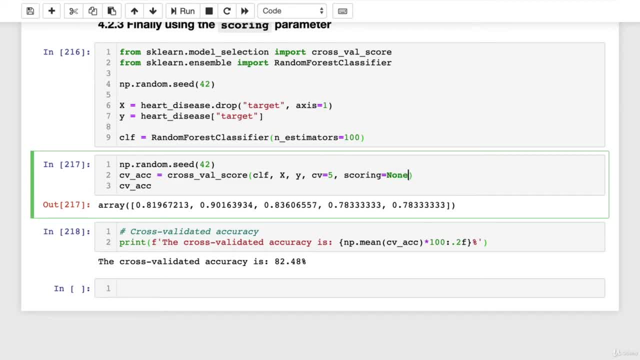 this is scoring equals none. so this is going to produce CVAC. and then if we go here- so now, if we just copy this right, actually what we might do is just test it out by only changing one thing. so if we take this, we'll copy this line just to prove it. this is where the scoring parameter. 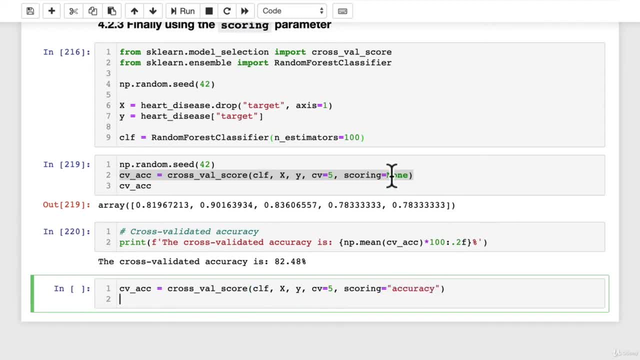 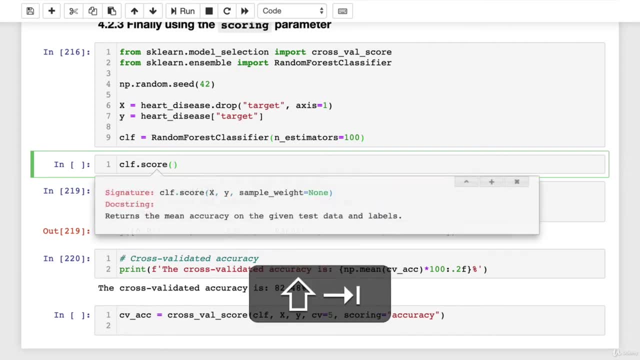 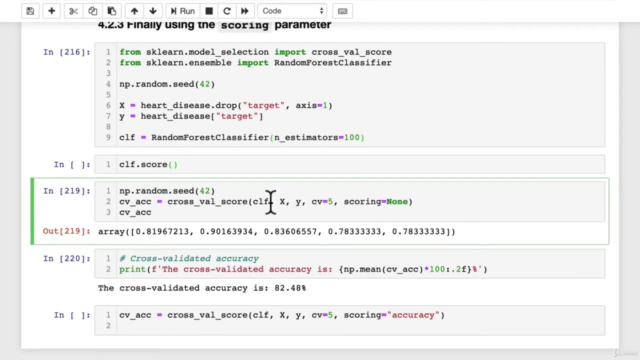 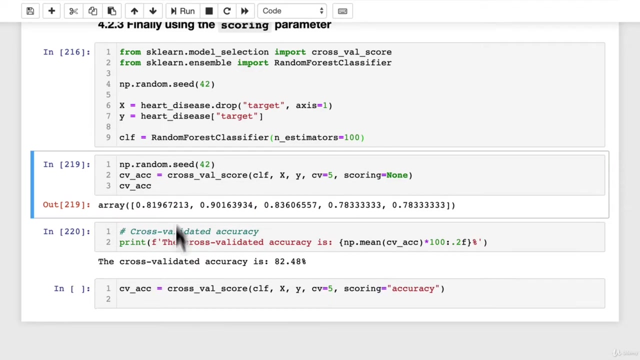 comes in so we can use accuracy here. all we're doing is changing none to accuracy because remember our random forest classifier by default uses mean accuracy, so remember the scoring parameter when left to none, uses a classifier or estimator's default parameter from score to evaluate using cross validation. so we'll get rid of that now. all we've done is 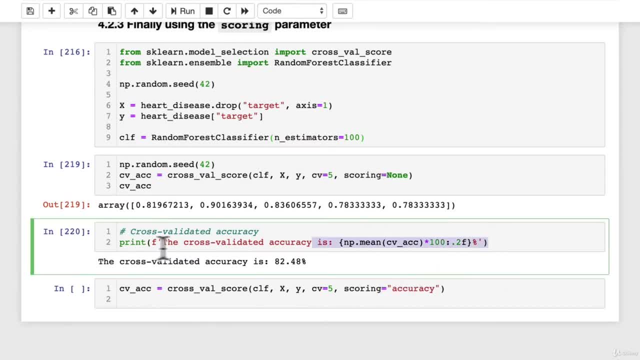 we've changed scoring equals accuracy, and then we're going to take this line here. we'll just copy this. and if this is true, then we're going to take this line here and we're going to copy this. it's true, right? if I'm not telling lies, it should print out the exact same thing here, because 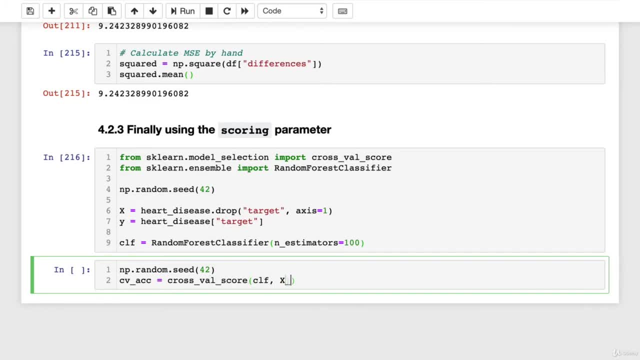 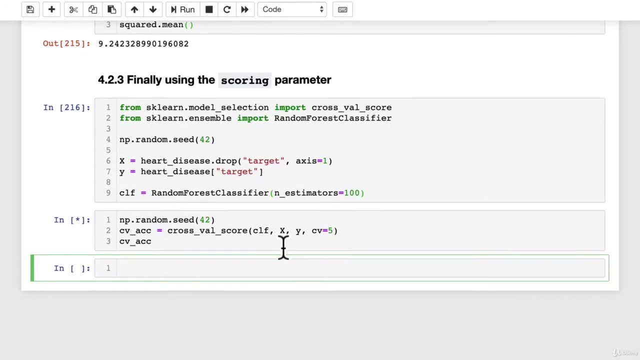 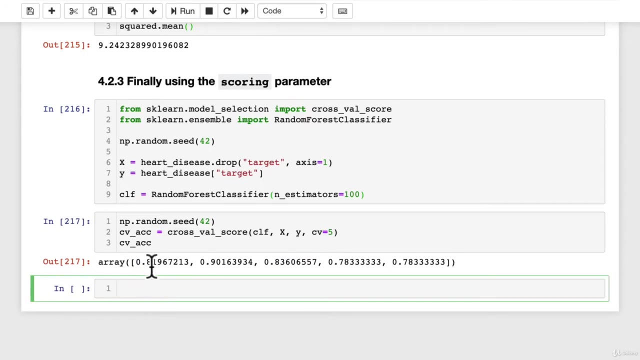 Cross-valScore, clf, x, y, and then we'll use five-fold cross-validation, cvac- Wonderful, It's going to train five models, evaluate them on different test sets, And then, of course, we could take the mean of this. 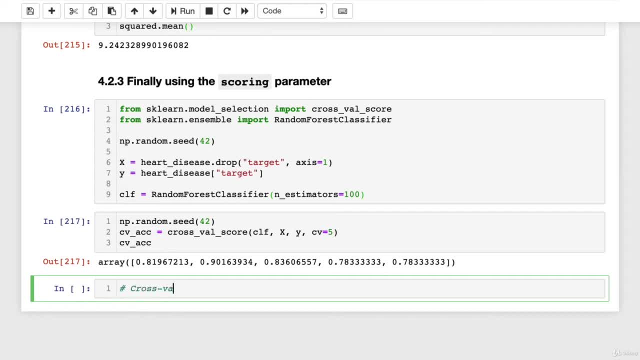 So why don't we do that? We'll go cross-validated accuracy, So we could go printf. The cross-validated accuracy is: I need some spaces here, Daniel. Come on The mean npmean cvac, And then we're. 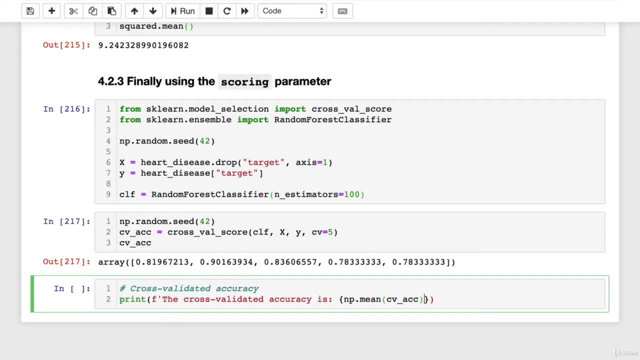 going to take that to. We'll only use cvac. And then we're going to take that to. We'll only use cvac. We'll only use times 100 and two decimal places And we'll put a little percentage sign on the end And we need a final string delimiter. Beautiful. So now the cross-validated. 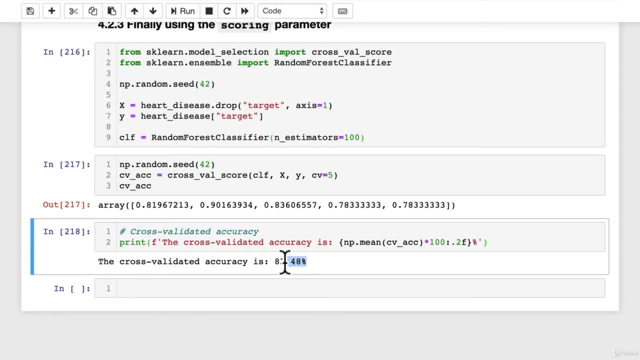 accuracy is 82.48%. Now, we've seen this before, right, We've seen this line. We've seen this line, And the reason why is we're using this is because, by default, the model it uses accuracy cross-valScore, because, in essence, this is: 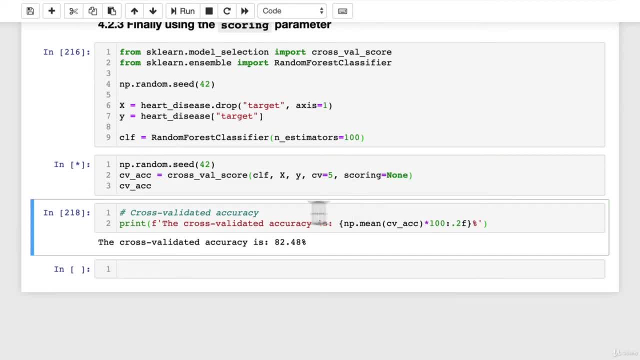 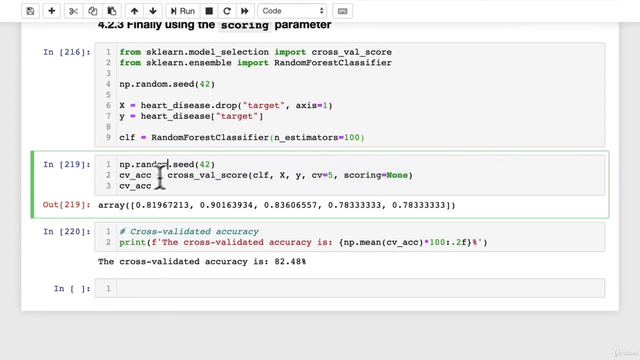 scoring equals none. so this is going to produce CVAC. and then if we go here, so now, if we just copy this right, actually what we might do is just test it out by only changing one thing. so if we take this, we'll copy this line, just to prove. 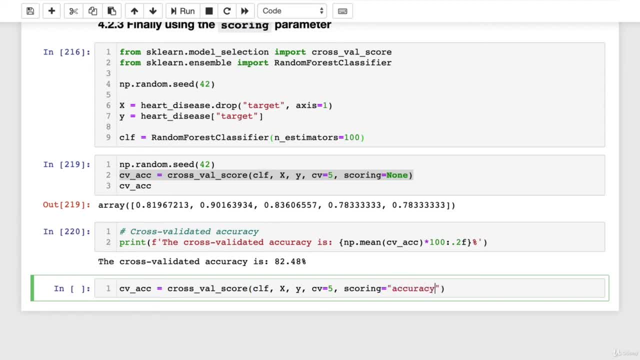 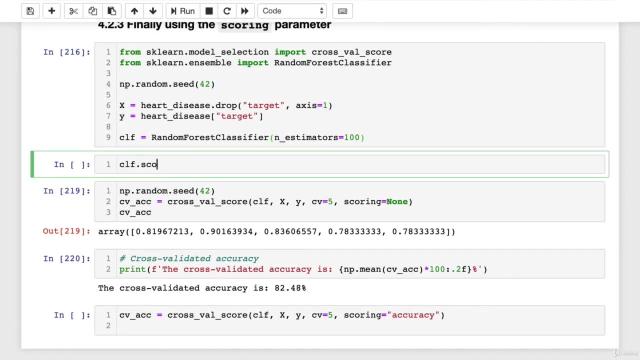 it. this is where the scoring parameter comes in, so we can use accuracy here. all we're doing is changing none to accuracy because remember our random forest classifier by default uses mean accuracy. so remember the scoring parameter when left to none, uses a classifier or estimators, default parameter from score. 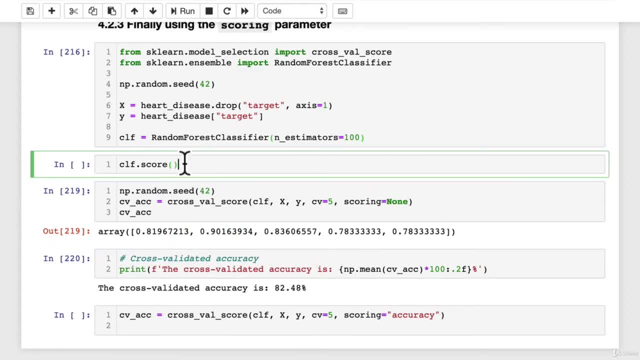 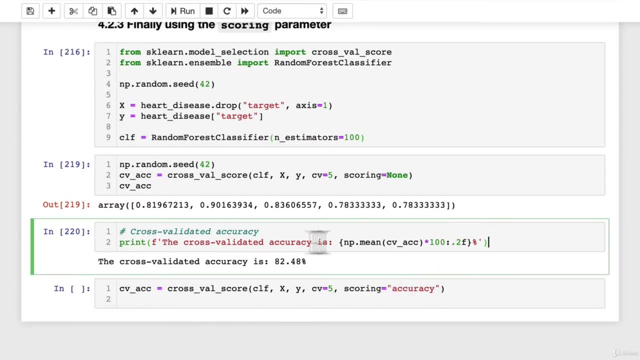 to evaluate using cross-validation. so we'll get rid of that. now, all we've done is we've changed scoring equals accuracy, and then we're going to take this line here: we'll just copy this and if this is true- right, if I'm not telling lies- it should print out. 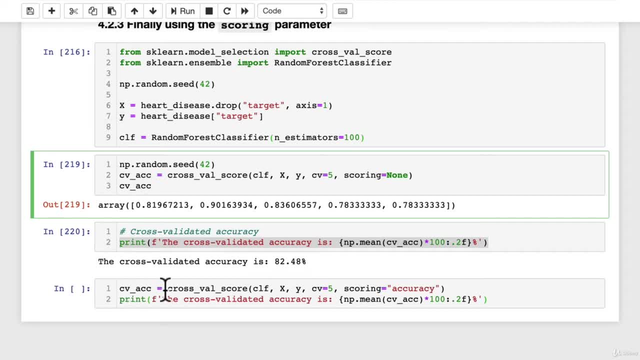 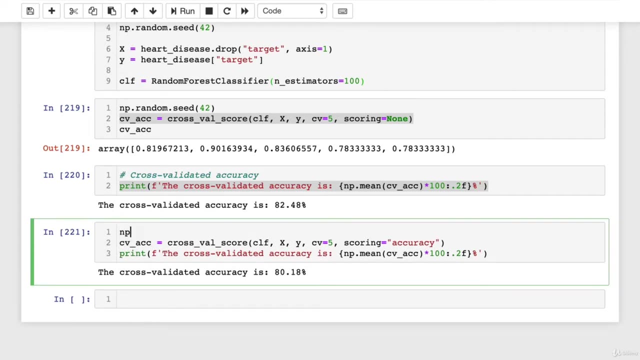 the exact same thing here, because CVAC equals cross-val score, CLF XY, CV equals five. scoring equals accuracy should be the same as this. well, let's see it. oh, you know why it was different was because we forgot our NP random seed. yes, there we go, boom. 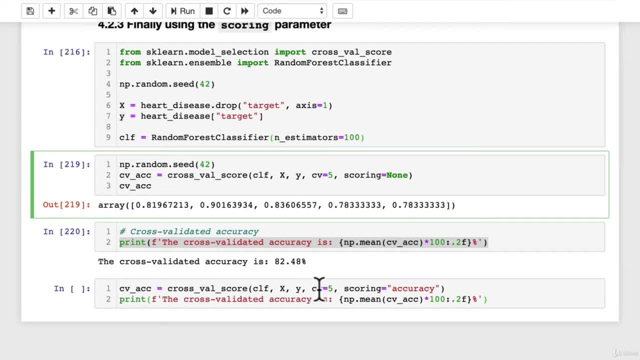 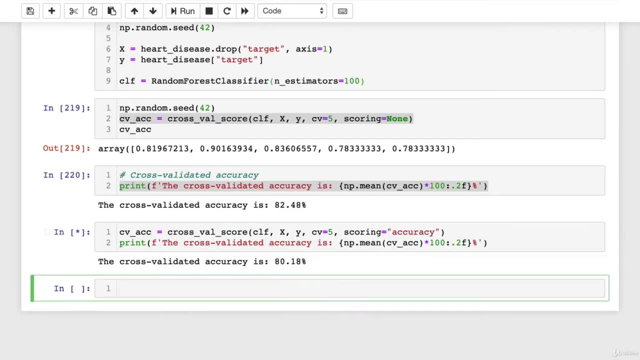 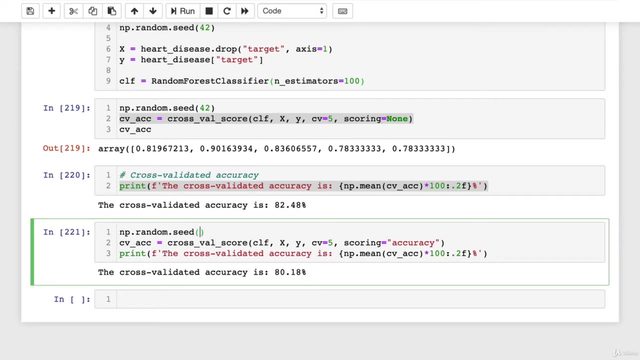 CVAC equals cross fail score. CLF, XY, CV equals five. scoring equals accuracy should be the same as this. let's see it. oh, you know why it was different was because we forgot our NP random seed. yes, there we go, boom see. that's another reason highlighting. 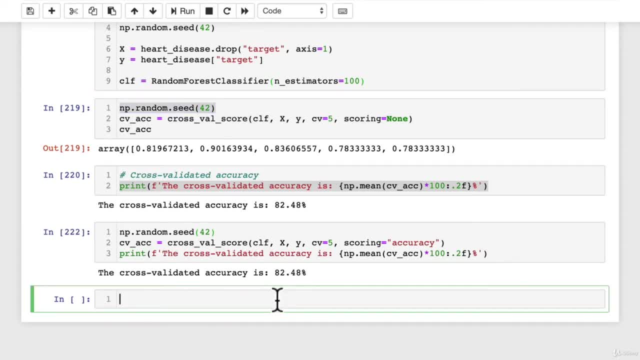 use of mp random seed right is making our experiments reproducible. all right, now to see another metric. this is where the scoring parameter really starts to shine. how about we use precision- so cv precision- to evaluate our classification model? cross val score? because, remember, precision is one of the metrics that we can use to evaluate our classification models. now, all we're going to 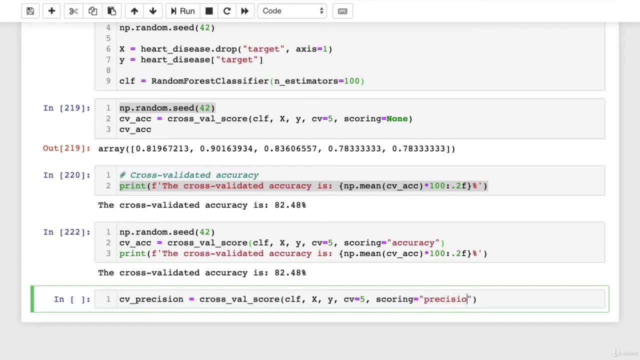 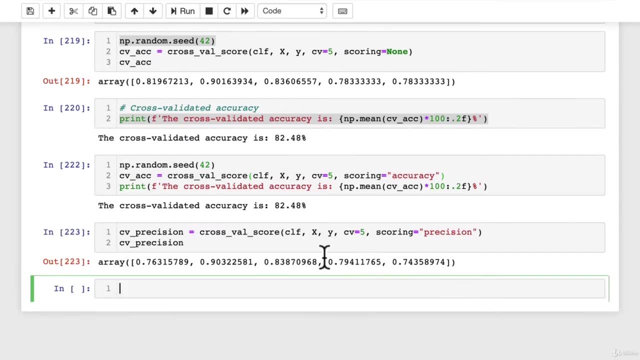 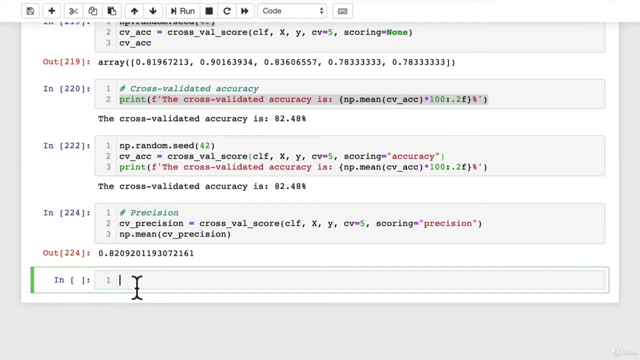 do is change scoring equal to precision, beautiful, and we'll see what cv precision is wonderful, but we probably take the np mean beautiful, so 0.82 on the precision front. we might do here precision. now. how about recall? so go, cv. recall equals cross val score, clf, x, y, cv equals five scoring. can you guess what? what the scoring? 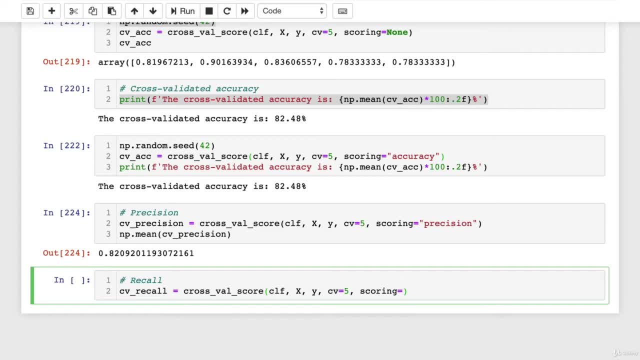 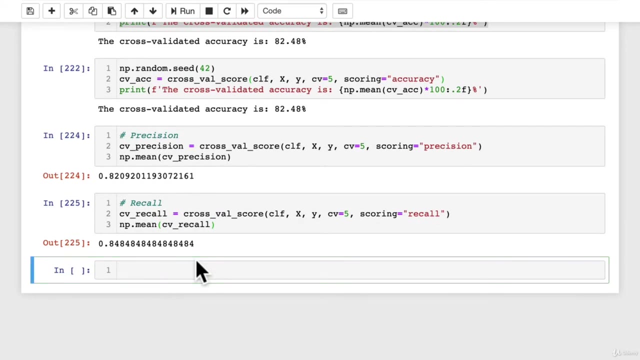 parameter might be equal to here if we wanted to calculate recall, not to worry, if you can't, we'll do it here. recall, and then we want np mean to get the cross validated recall. wonderful 0.84 recall. and now, how about for f1? how about we do that? yeah, why not cv f1? 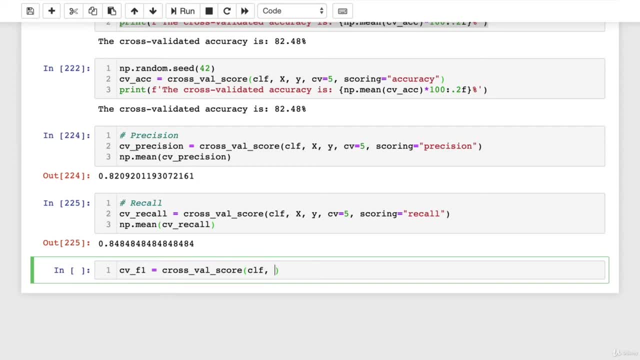 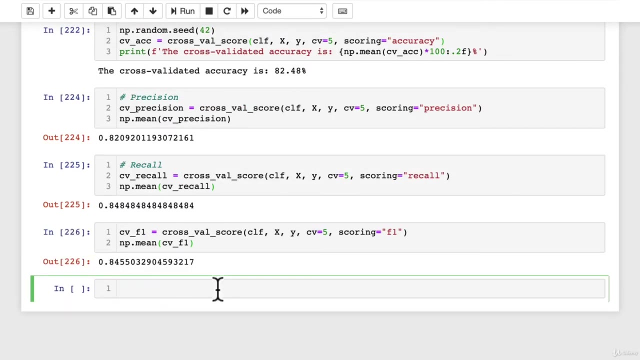 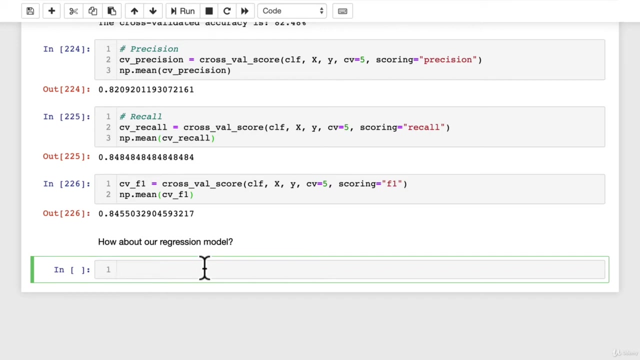 equals. remember, f1 is a combination of precision and recall. x, y, cv equals five. scoring equals f1. we want np mean dot, cv, f1. wonderful, there we go. okay, now we've done some classification metrics here. how about our regression model? well, Why don't we make a regression model and check it out? 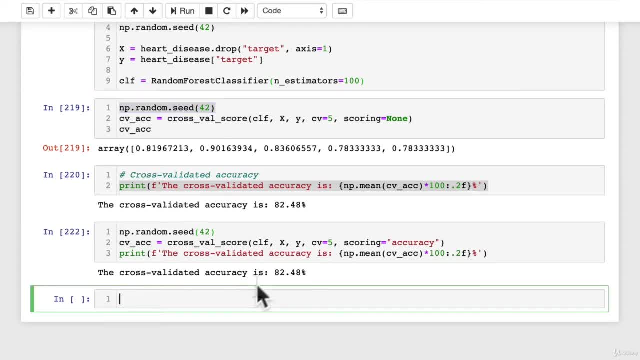 see. that's another reason. highlighting the use of NP random seed right is making our experiments reproducible. all right, now to see another metric. this is where the scoring parameter really starts to shine. how about we use precision- so CV precision- to evaluate our classification model? cross-val score. 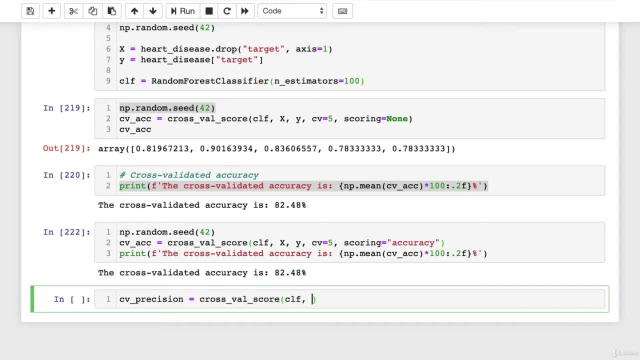 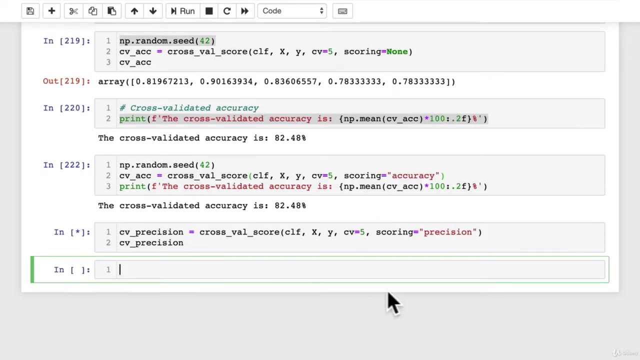 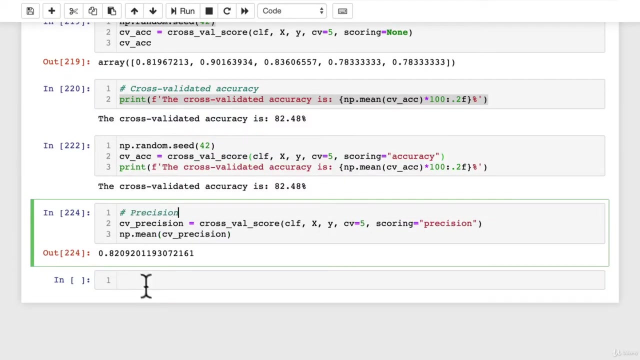 because, remember, precision is one of the metrics that we can use to evaluate our classification models. now, all we're going to do is change scoring equal to precision beautiful, and we'll see what CV precision is wonderful, but we probably take the NP mean beautiful. so, point 82 on the precision front, we might do here: precision now how? 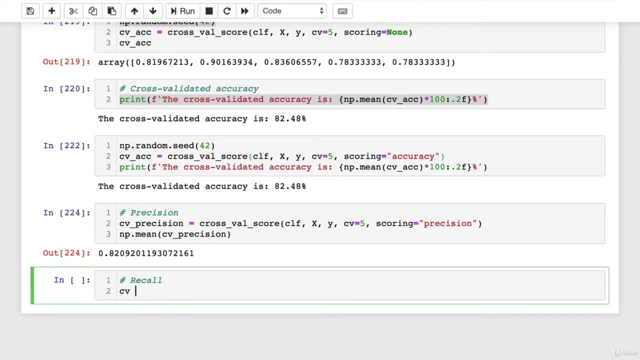 about recall. so go. CV. recall equals cross-val score, CLF XY. CV equals 5 scoring. can you guess what the scoring parameter might be equal to here if we wanted to calculate recall? not to worry, if you can't, we'll do it here. recall and then we want NP mean to get 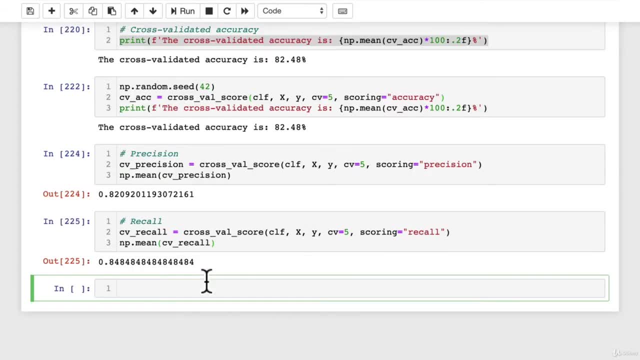 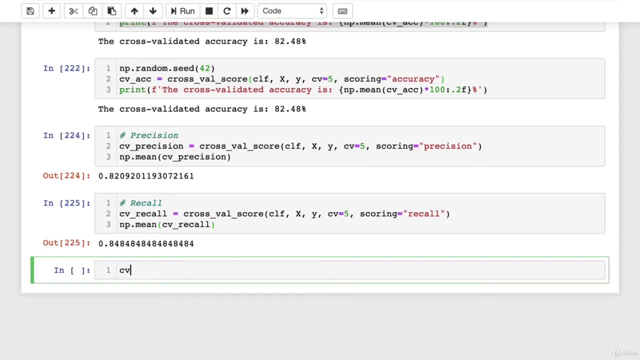 the cross validated recall. wonderful 0.84 recall. and now, how about for F1? how about we do that? yeah, why not? CVF1 equals, remember, F1 is a combination of precision and recall. XY CV equals 5, scoring equals. 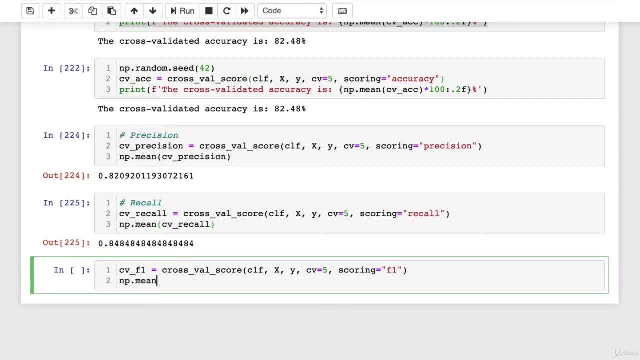 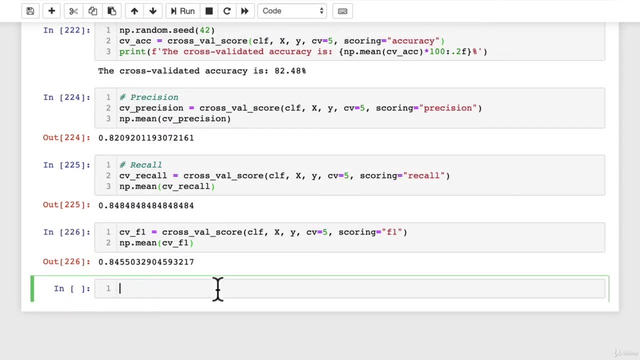 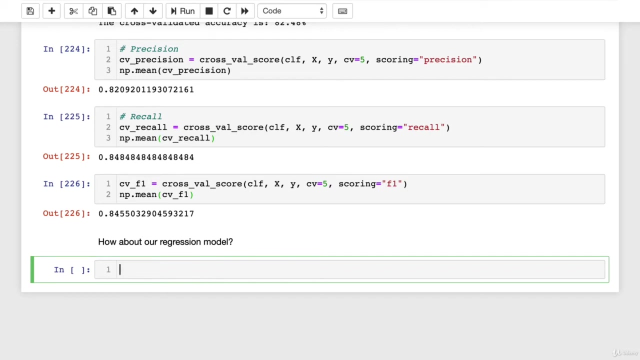 F1, we want NP mean CVF1. wonderful, there we go. ok, now we've done some classification metrics here. how about our regression model? well, why don't we make a regression model and check it out? ok, from sklearnmodelselection. 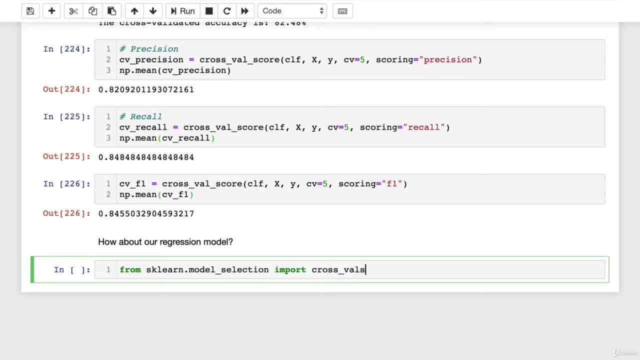 import crossval score. so we want to cross validate our regression model's predictions. so from sklearnensemble to get all the benefits that cross validation offers. random forest regressor. look at us. go typing machine learning code like it's nothing. go NP, random seed 42. 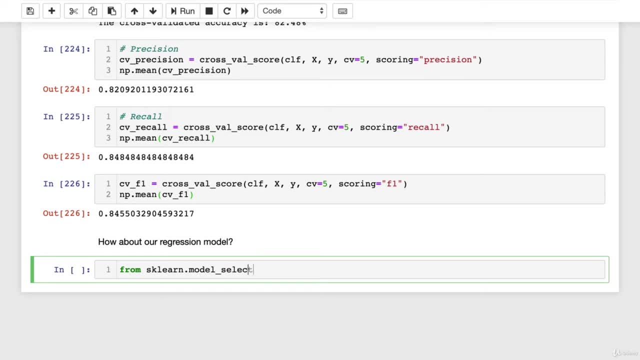 Okay, From sklearnmodelSelection import crossValScore. So we wanna cross validate our regression model's predictions. So from sklearnensemble to get all the benefits that cross validation offers. Random forest regressor. Look at us go Typing machine learning code like it's nothing. 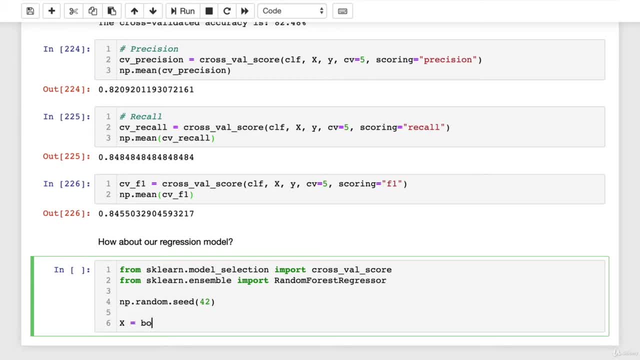 We go np, random seed 42. We'll create our x data. So boston df. Yes, drop target Axis. can you guess what axis Axis equals one? yes, Equals boston df. So this is y actually Target. I'm getting ahead of myself. 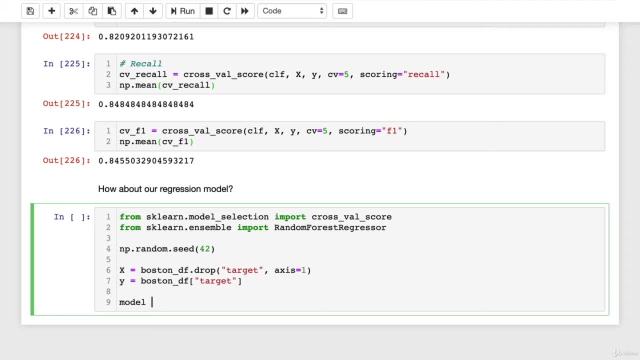 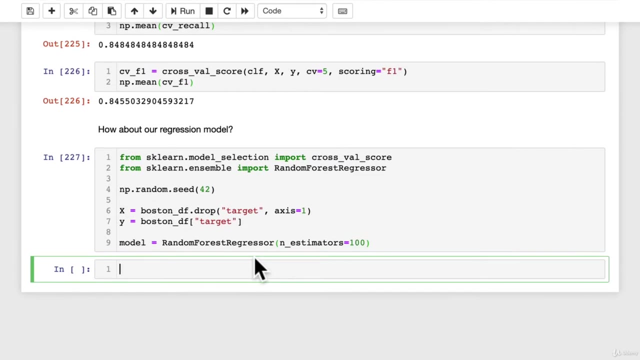 My voice can't keep up with my coding Model equals- which is very unusual for me, actually, Random forest regressor. We'll set n estimators again to being tab, autocomplete to being 100.. Wonderful, And now do you remember what the default metric is? 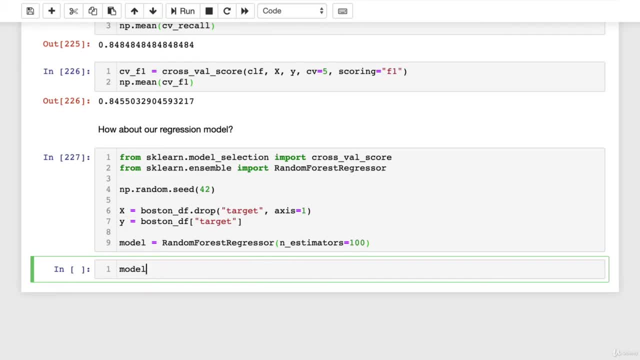 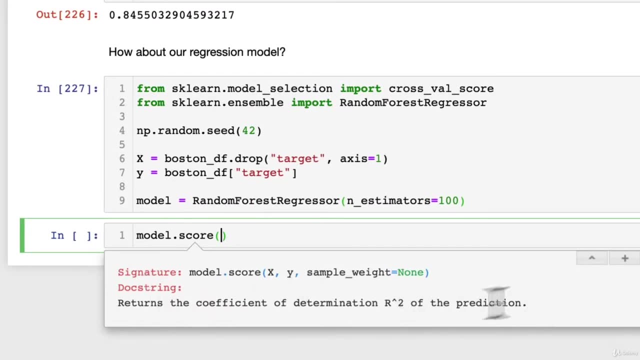 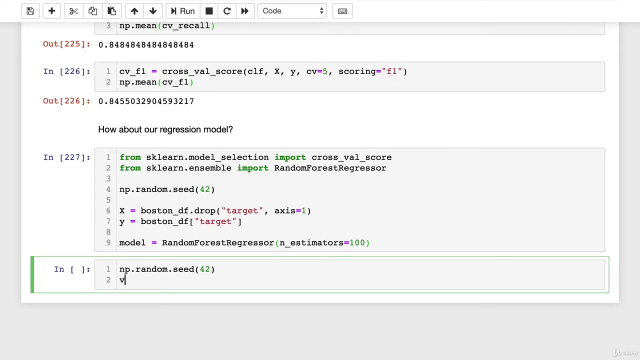 for score for a regression model. So if we do modelscore, the default evaluation metric is: returns, the coefficient of determination, r squared of the prediction. Alrighty, Well, let's check it out. So np, random seed, And then we're gonna go cv: r squared equals crossValScore. 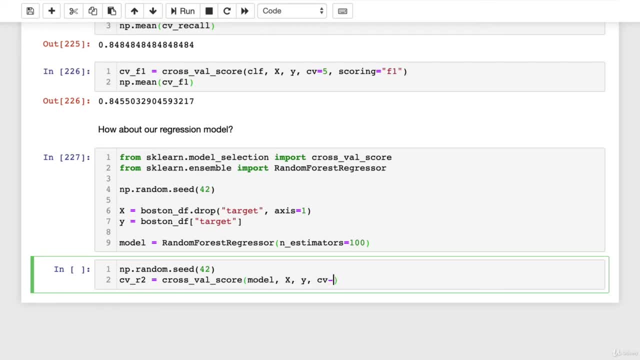 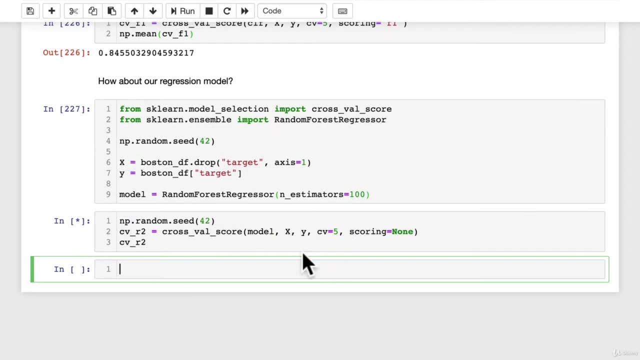 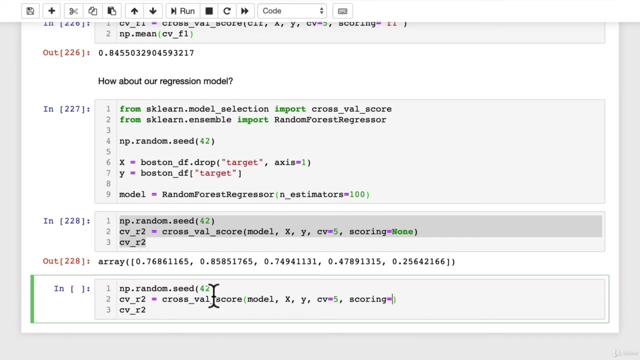 Model, this time x, y, cv, five-fold cross validation. Let's do scoring equals none, Right? and then we're gonna cv r squared And we're gonna copy this exact code: Boom, And because, remember, crossValScore uses. 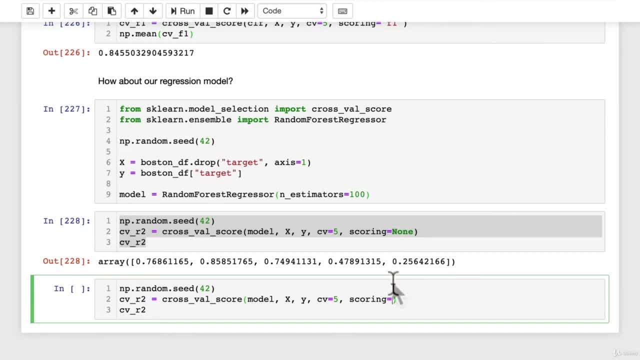 the default evaluation metric in the score function if set to none. So if we just change this to be r2, what do you think is gonna happen? Because this is surefire. So if we just change this to be r2, what do you think is gonna happen? 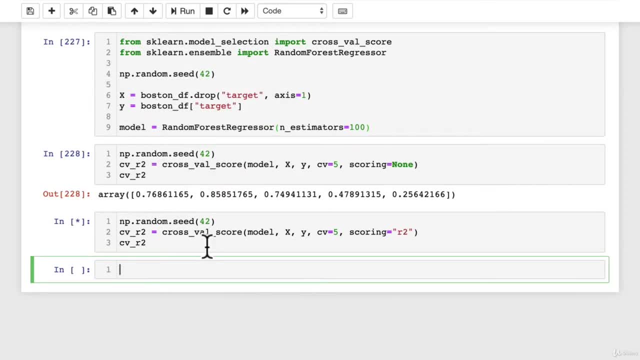 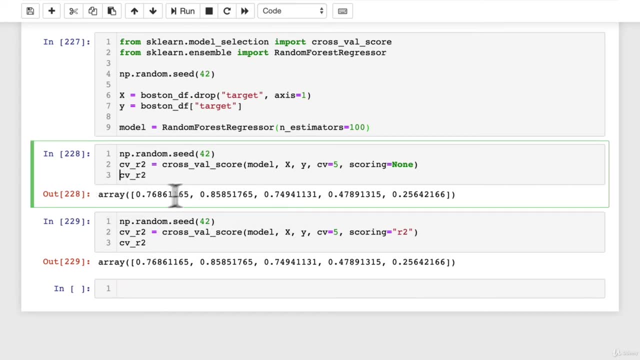 Because this is sure for r squared right. So if we go here, boom, we get the same values. Look at this Now. this is pretty drastically different, right? So we got over here. this is 0.85.. This is what I was talking about in getting that lucky split. 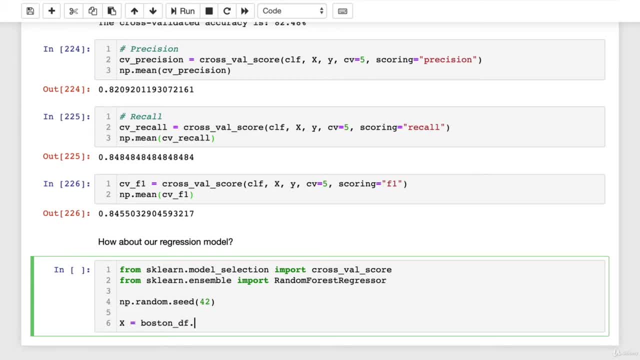 we'll create our X data. so BostonDF: yes, drop target axis. can you guess what axis axis equals 1, yes, equals BostonDF. so this is Y actually target. I'm getting ahead of myself. my voice can't keep up with my coding. 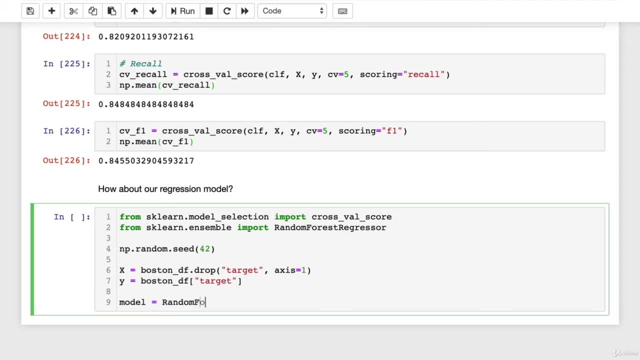 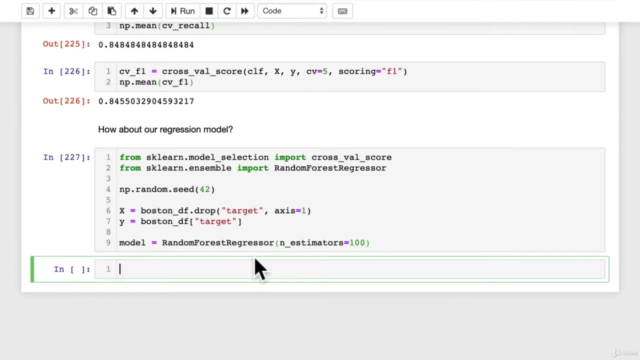 model equals- which is very unusual for me- actually random forest regressor. we'll set N estimators again to being tab autocomplete, to being 100, wonderful. and now do you remember what the default metric is for score for a regression model? so if we do modelscore, 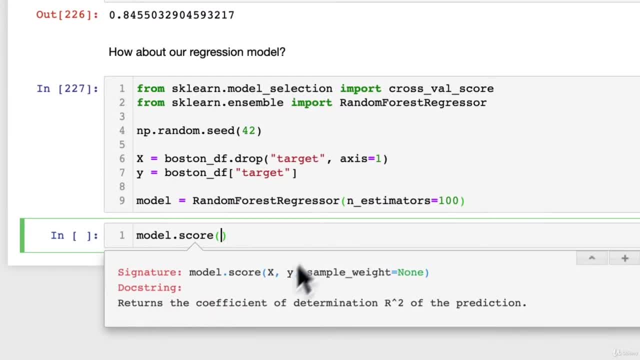 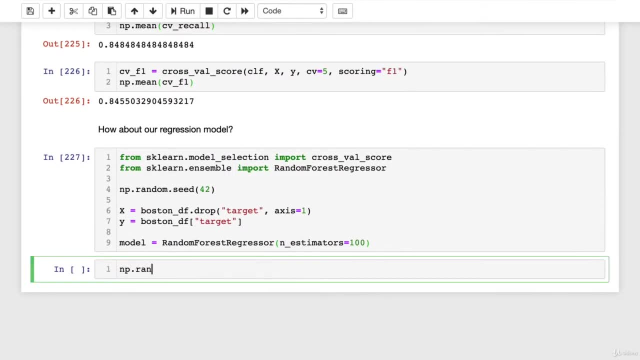 the default evaluation metric is: returns, the coefficient of determination, R squared of the prediction. alrighty, well, let's check it out. so NP, random seed, and then we're gonna go: CV, R squared equals cross val score model, this time X, Y, CV, five fold cross validation, let's do: scoring equals none. 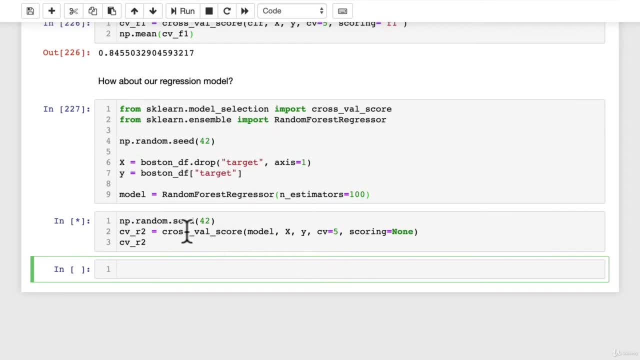 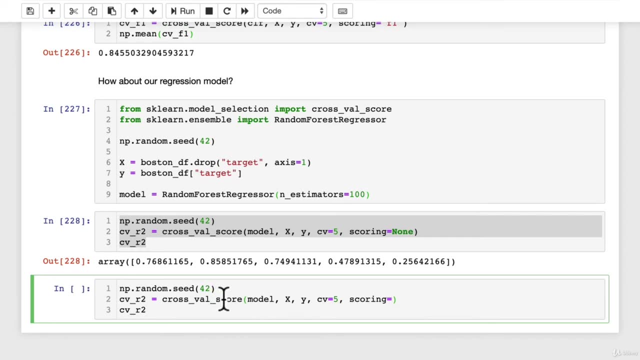 right. and then we're gonna CV R squared and we're gonna copy this exact code. boom. and because, remember, cross val score uses the default evaluation metric in the score function if set to none. so if we just change this to be R2, what do you think's gonna happen? 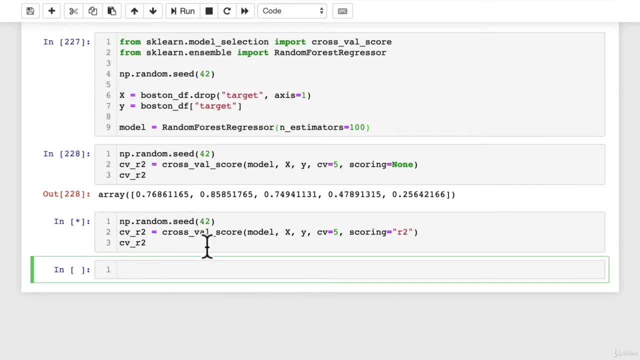 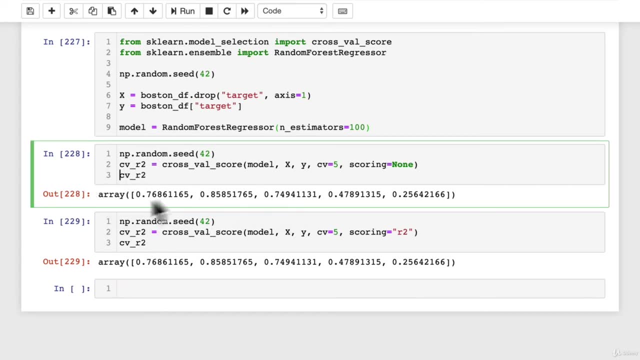 because this is short for R- squared right, squared right. So if we go here, boom, We get the same values. Look at this Now. this is pretty drastically different, right? So we've got over here. this is 0.85.. This is what I was talking. 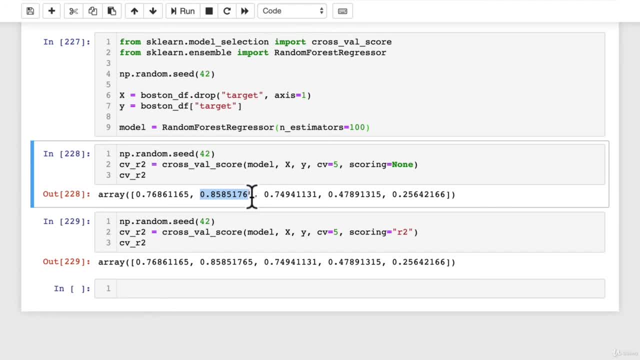 about getting that lucky split. So cross validation: on this one it's done pretty well, So 0.85. But on this split it's only done 0.25.. So if we got here, if we did, the MP mean 0.622.. Now that's quite a bit different to the first. 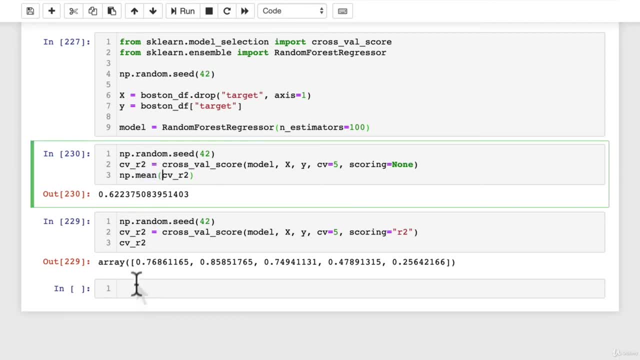 R squared score. we saw just using the score function. Well, let's keep going, Let's not stop there. How about we do mean absolute error, because that's another regression metric. So let's try it out. So, CVMAE, We'll put it in here. 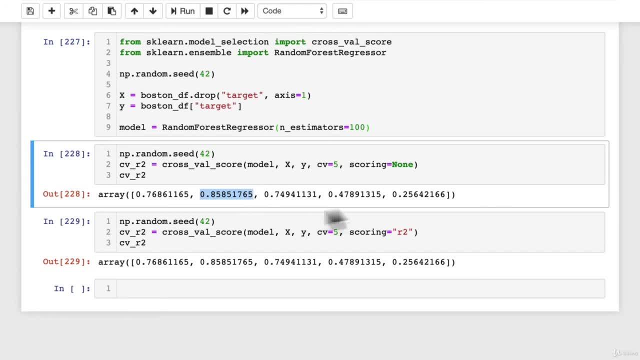 So cross validation: on this one it's done pretty well, So 0.85.. But on this split it's only done 0.25.. So if we got here, if we did the np, mean it's 0.622. 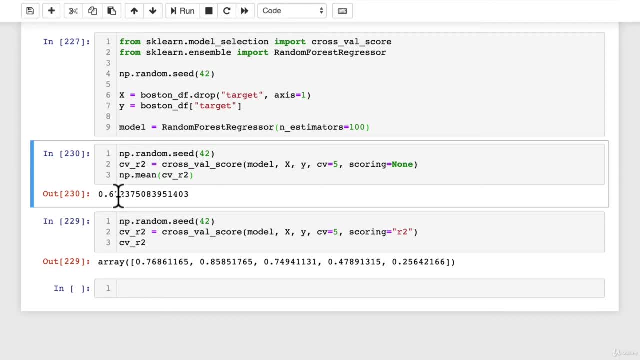 Now that's quite a bit different to the first r squared score we saw just using the score function. Well, let's keep going, Let's not stop there. How about we do mean absolute error, because that's another regression metric. So let's try it out. 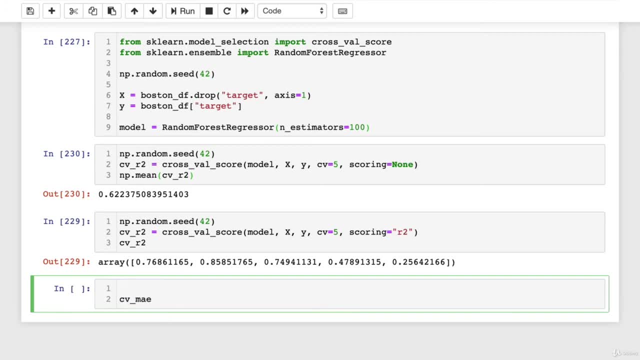 So cvmae- we'll put it in here- Mean absolute error. Wonderful, cvmae equals crossValScore. We'll pass it. our model, which is a random forest regressor, x, y, a cv of five Scoring is going to be: 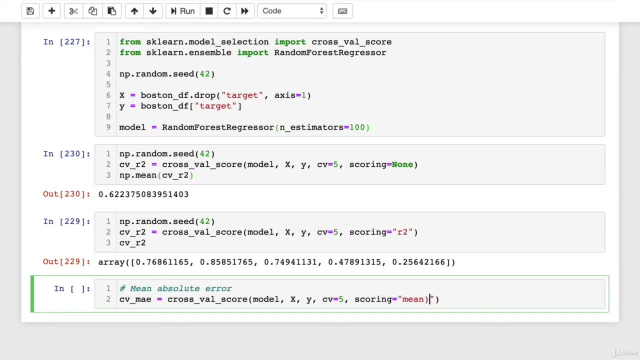 hmm, what might this be? We might type in, we'll guess this string mean absolute error. Let's just see them all laid out, because that was pretty cool to see with our r squared score, right, Just to see how different they can be. 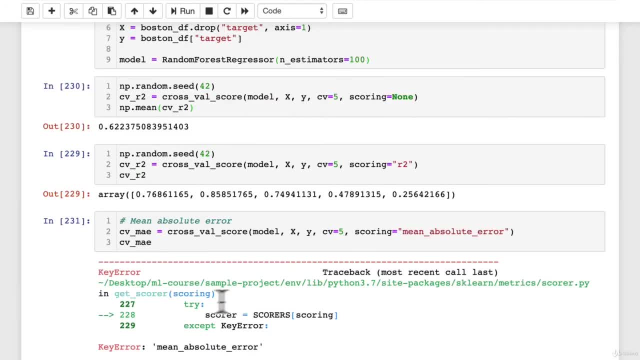 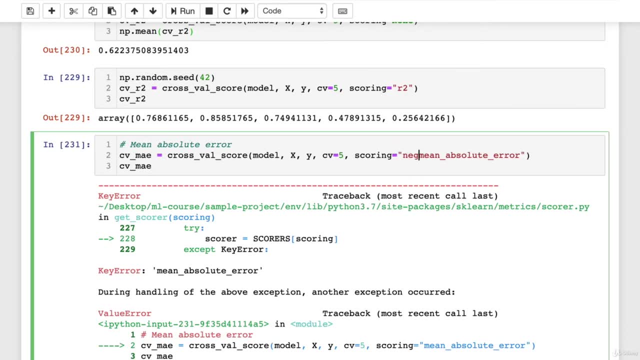 across five different splits of data using cross validation. Key error mean absolute error. Now why is that? And I'll tell you why. It's because we need neg in the front here. Oh, and you might be asking again: why neg? 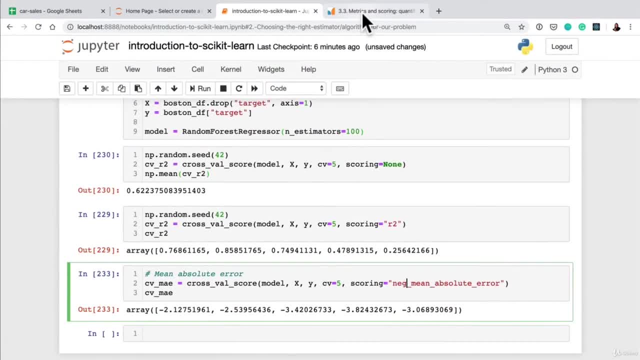 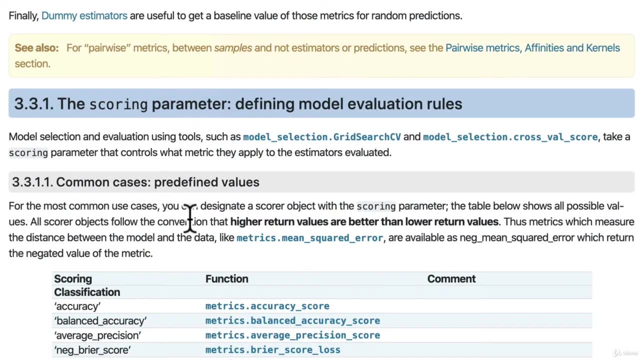 But I'll show you that in a second. Okay, so that's interesting. So if we come up here, we can tell why it means. neg is because all score objects follow the convention that higher return values are better than lower return values, right? 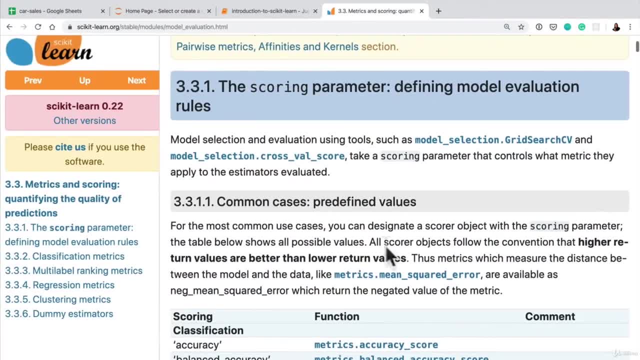 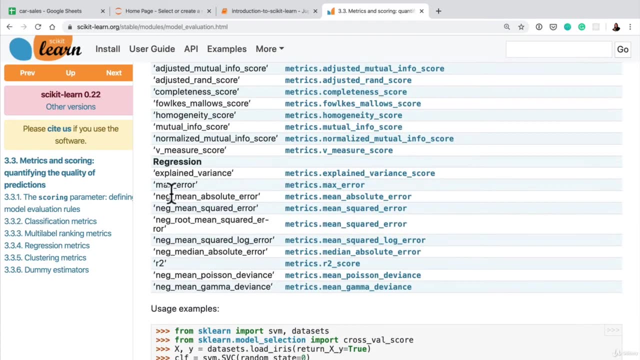 So that's a key point to remember here. This is in the documentation. All score objects follow the convention that higher return values are better than lower return values. So if we come down here, this is why we have might zoom out, because that's looking a bit too big. 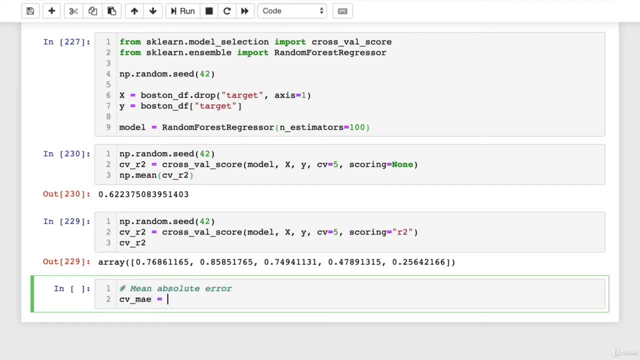 Mean absolute error. Wonderful CVMAE equals cross of our score. We'll pass it our model, which is a random forest regressor, XY a CV of 5. Scoring is going to be: hmm, what might this be? We might type. 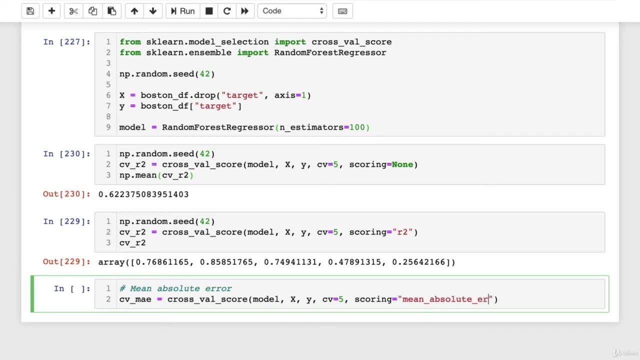 in we'll guess this string mean absolute error. Let's just see them all laid out, because that was pretty cool to see with our R squared score right, Just to see how different they can be across five different splits of data using cross validation. 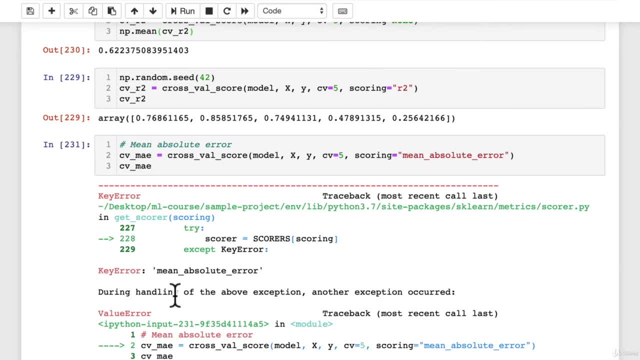 Key error Mean absolute error. Now why is that? And I'll tell you why. It's because we need neg in the front here. And you might be asking again, why neg? But I'll show you that in a second. Okay. 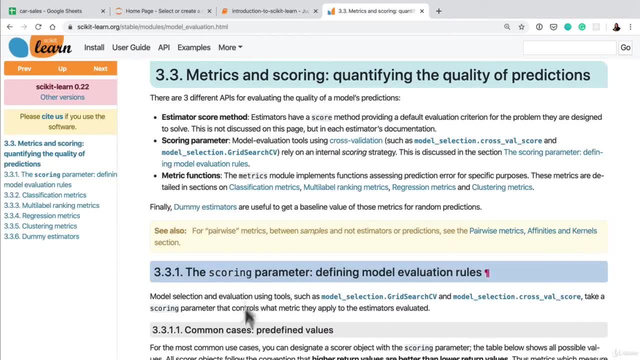 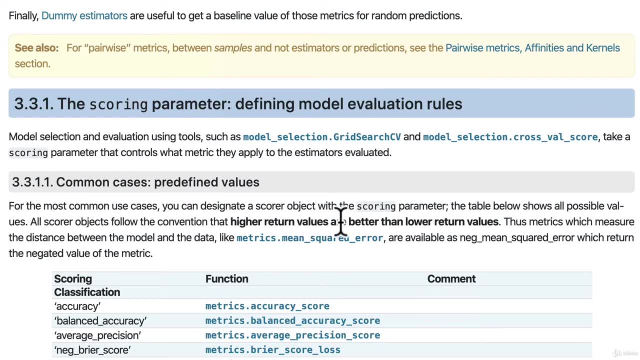 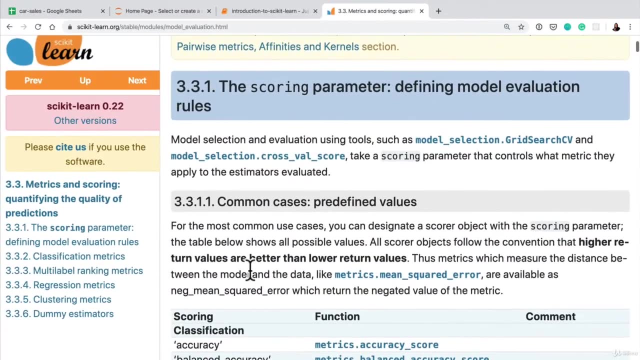 So that's interesting. So if we come up here we can tell why it means. neg is because all scorer objects follow the convention that higher return values are better than lower return values, Right? So that's a key point to remember here. This is in the documentation. 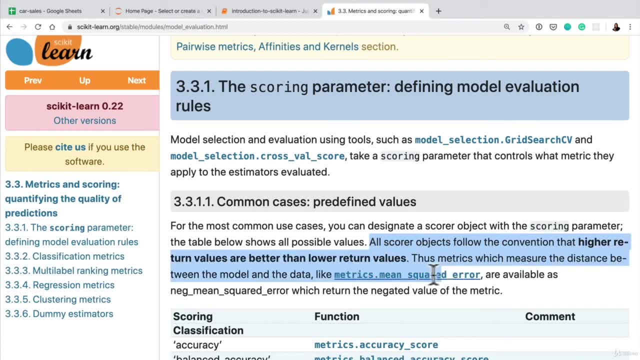 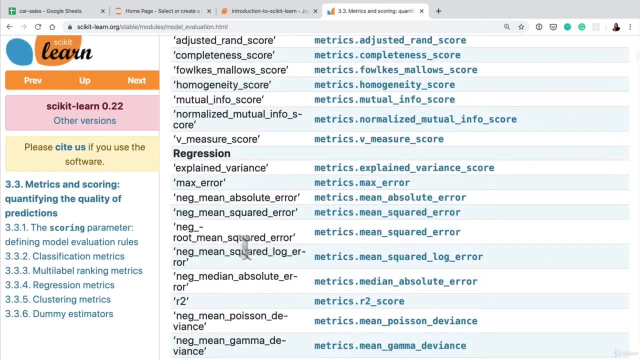 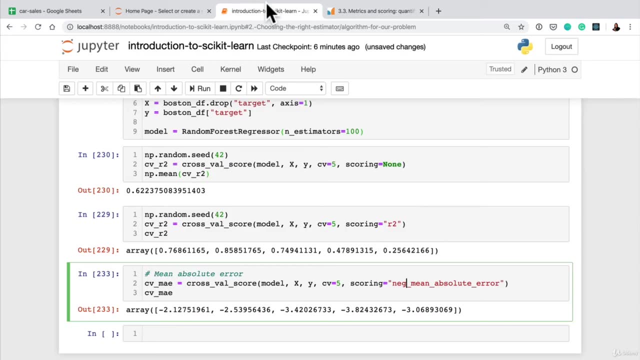 All scorer objects follow the convention that higher return values are better than lower return values. So if we come down here, this is why we have might zoom out, because that's looking a bit too big. This is why we have neg mean absolute error. I'm looking back in our notebook. See these: 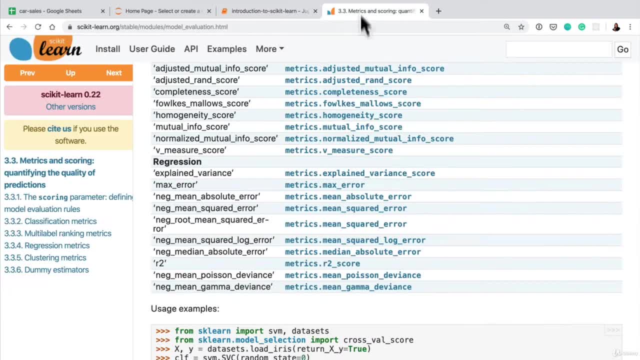 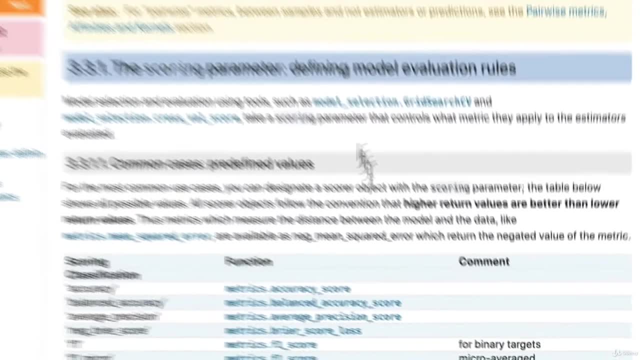 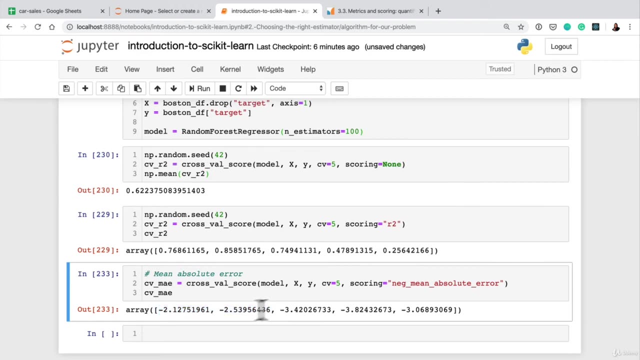 values are all negatives, And the reason being is because all scorer objects follow the convention that higher return values are better than lower return values. So that means, because these are negative, the higher these are, so the closer they are to zero it's better than the lower they are. So these are pretty low, So again, 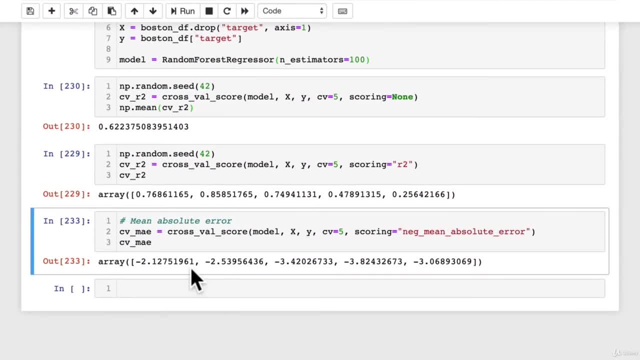 our model isn't perfect, But you can see the variations in the mean absolute error values, just like we had in the R-squared values. is that some splits right? because we did five splits are offering negative .212.. We saw 2.12 up before, But other ones are getting. we're getting. 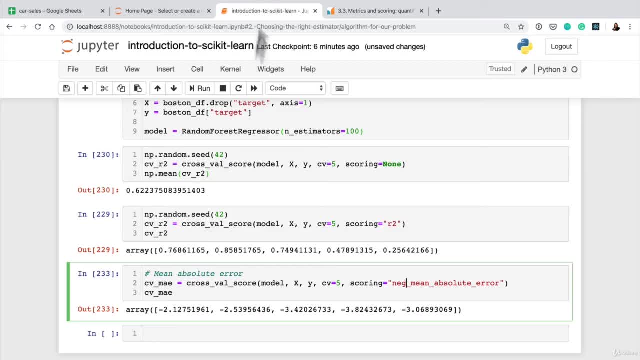 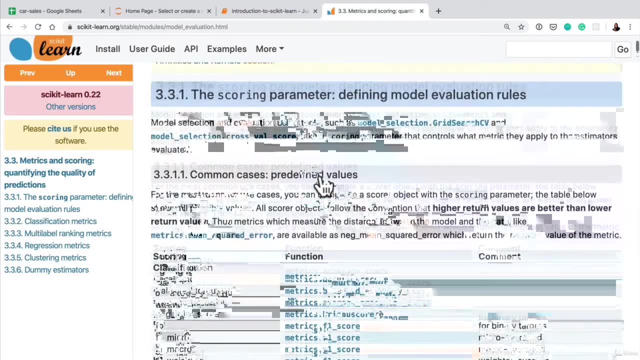 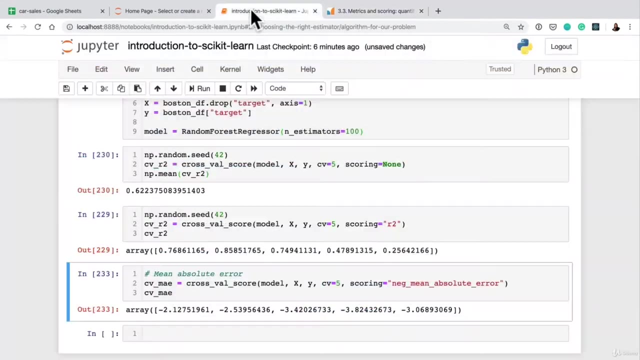 This is why we have neg mean absolute error. I'm looking back in our notebook. See, these values are all negatives And the reason being is because all score objects follow the convention that higher return values are better than lower return values. So that means because these are negative. 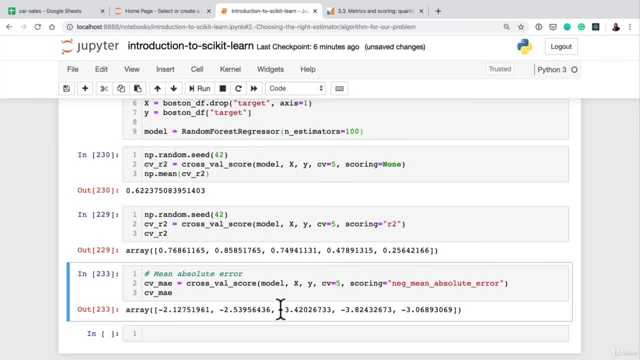 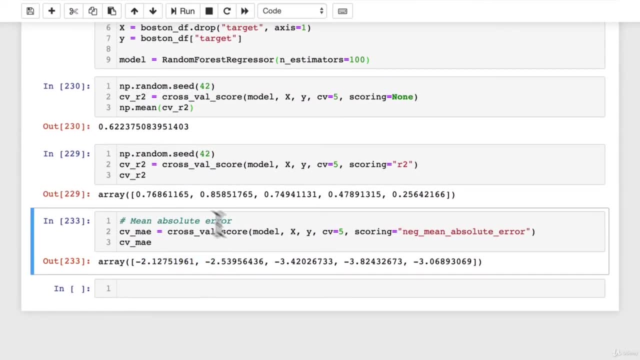 the higher these are, so the closer they are to zero it's better than the lower they are, So these are pretty low. So again, our model isn't perfect, but you can see the variations in the mean absolute error values, just like we had in the R squared values. 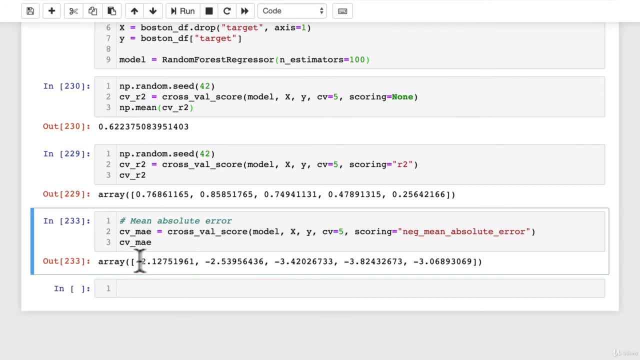 Is that some splits- right- Cause we did five splits- are offering negative 0.212.. We saw 2.12 up before, but other ones are getting. we're getting a much higher one here, So negative 3.8.. 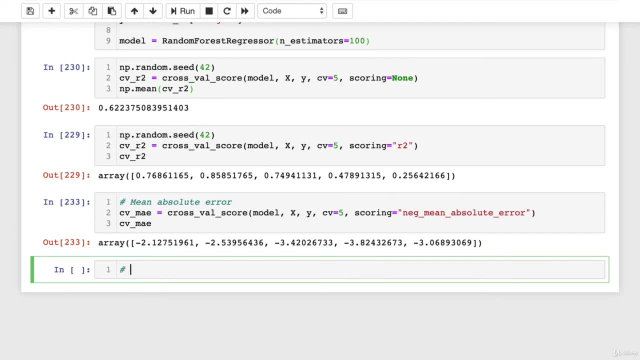 So this is where cross validation really comes into play. right Is figuring out. okay, are we just getting a lucky split on our model and training it on some easy training data to understand And then evaluating on the test data set? we might be going if it's a lucky split. 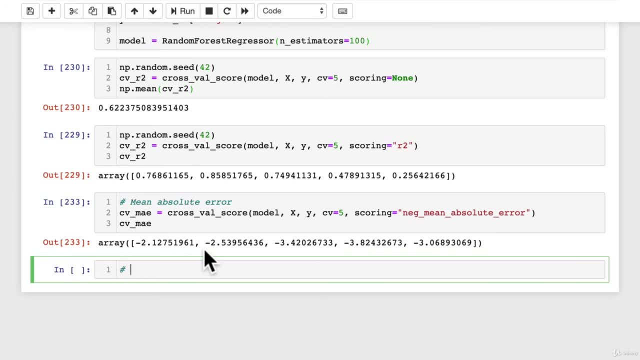 it might be getting metrics that aren't really congruent with how the model is actually performing. So let's finish this off. We're doing mean squared error, And now I bet you can guess how to do this one. So CV MSE equals MSE for mean squared error. 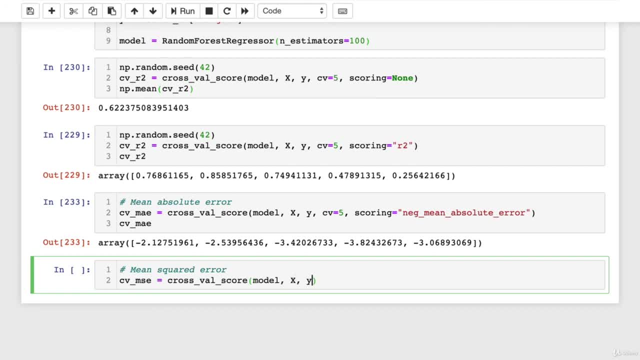 Cross val score. we'll pass it the model, And then do X, Y and we'll do CV equals, five, Scoring equals. Now if we'd had to do neg, mean absolute error, what do you think it is for? mean squared error. 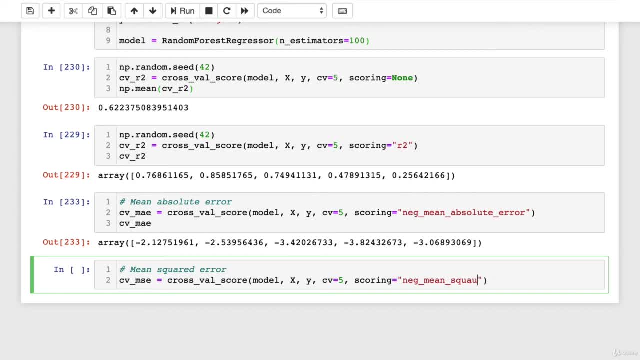 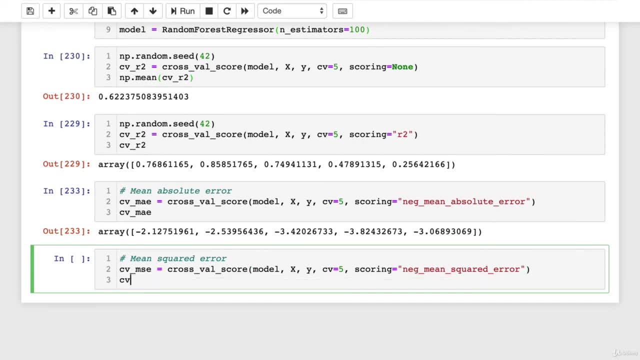 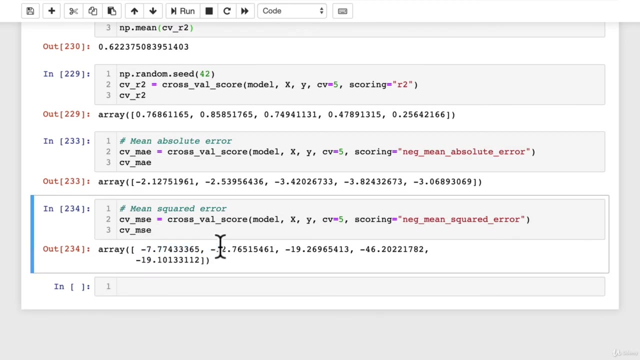 And if you guessed, neg mean squared error, you would be 100% correct, which is the opposite to what our model is: CV, MSE, Shift and enter, And again we're seeing some quite quite a wide range of values here, right? 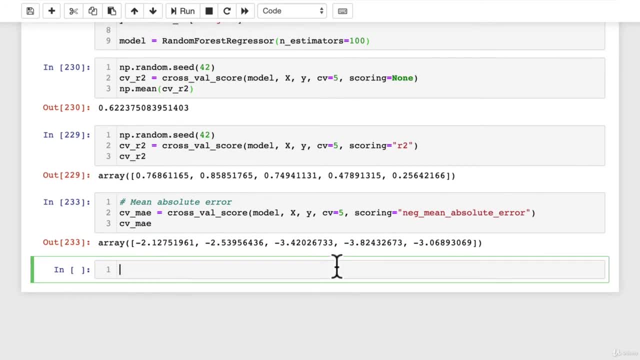 a much higher one here, so negative 3.8.. So this is where cross-validation really comes into play. right, It's figuring out okay, are we just getting a lucky split on our model and training it on some easy training data to understand? 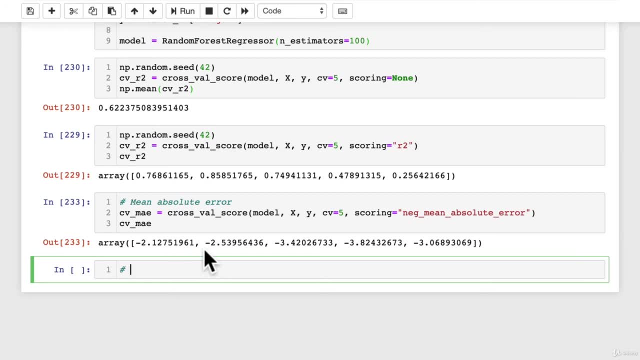 And then evaluating on the test data set we might be going. if it's a lucky split, it might be getting metrics that aren't really congruent with how the model is actually performing. So let's finish this off. We're doing mean, squared error. 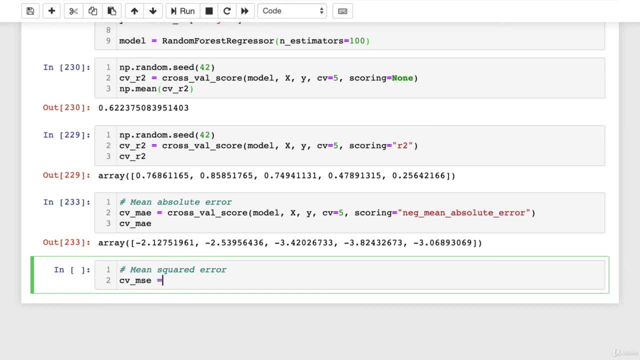 And now I bet you can guess how to do this one. So CVMSE equals MSE for mean squared error, Cross-val score. we'll pass it, the model, And then do XY and we'll do CV equals 5.. Scoring equals. 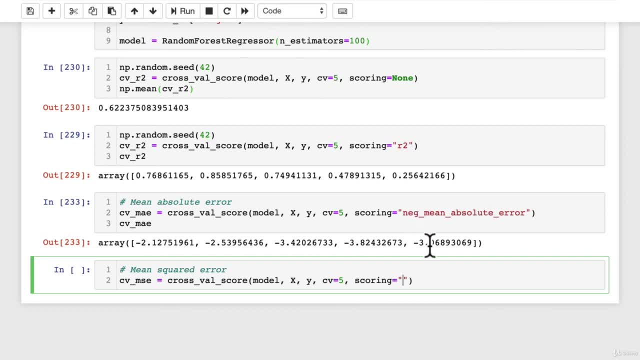 Now, if we'd had to do, neg mean absolute error. what do you think it is for? mean squared error? And if you guessed neg mean squared error, you would be 100% correct, which is the opposite to what our model is. 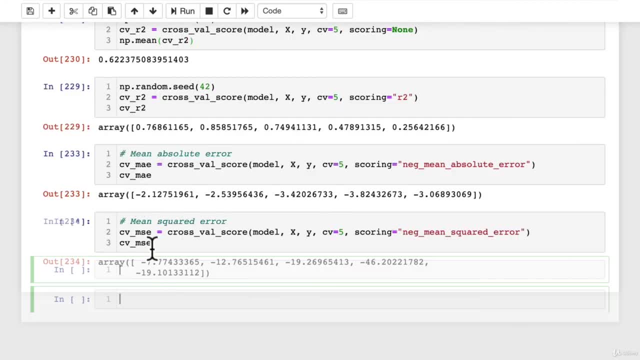 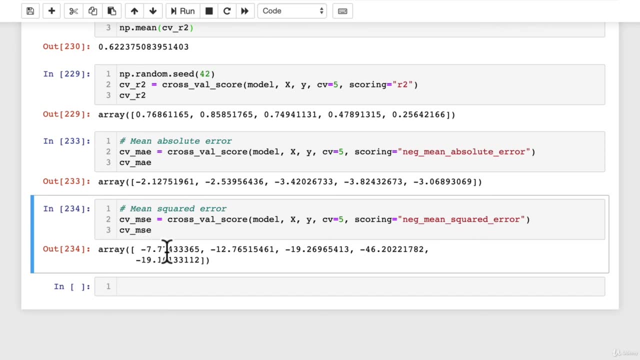 CVMSE, Shift and enter. And again we're seeing quite a wide range of values here, right. So we go from negative 7.77 right up to the highest one here is negative 46.2.. So we could take the mean of these to see. 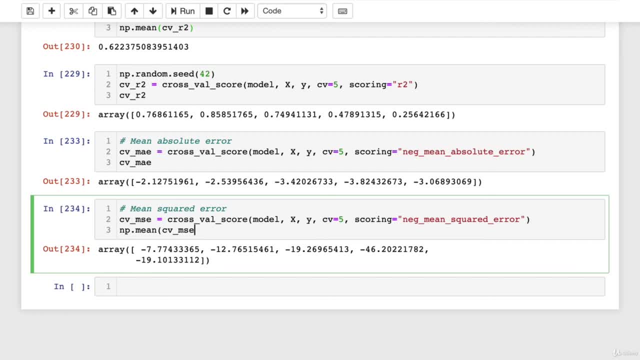 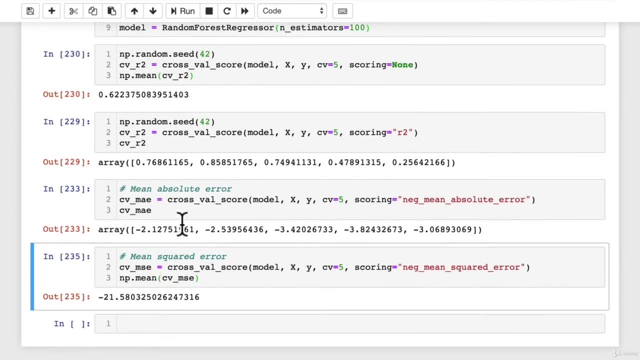 what it looks like across five different splits. So negative 21.5.. So that's a bit different again to our previous value, when we weren't using cross-validation right of mean squared error is 9.24.. Hmm, 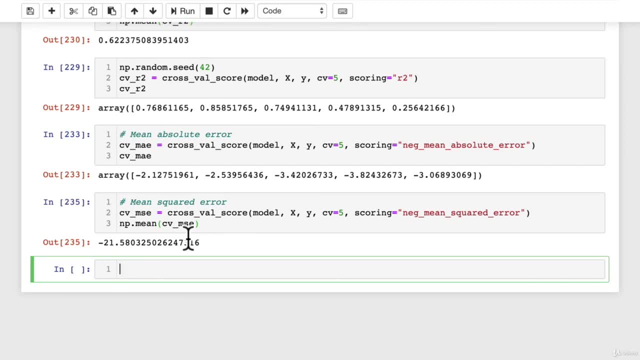 So, naturally, if we're looking at these evaluation metrics and we're starting to see, okay, we want to get better metrics, you might be starting to think is like, how can we start to improve these metrics, How can we make them better? 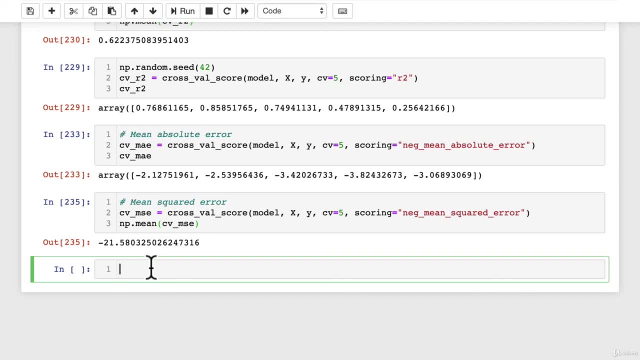 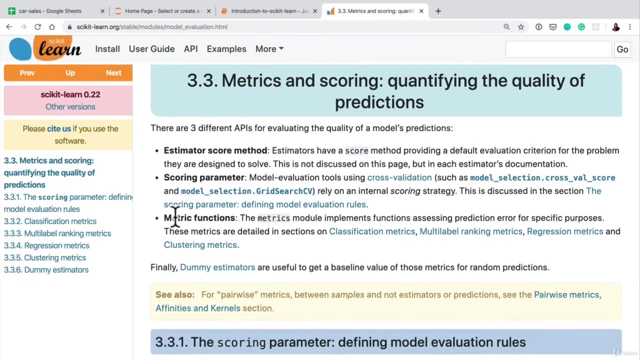 And we're definitely going to look at that. But finally, to finish the evaluation metric section off, we're going to have a look at the third and final way of evaluating a model, and that is using metric functions. Spoiler alert: you've seen some of these in action before. 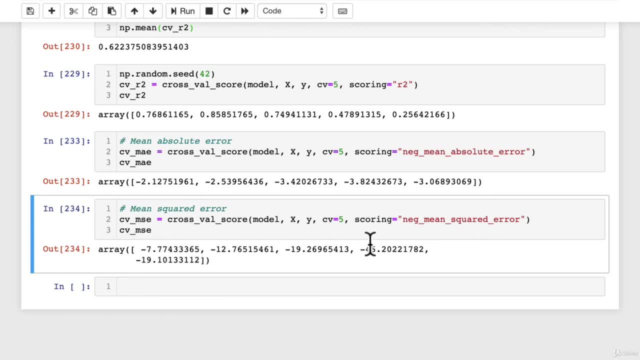 So we go from negative 7.77, right up to the highest one here is negative 46.2.. So we could take the mean of these to see what it looks like across five different splits. So negative 21.5.. So that's a bit different again to our previous value. 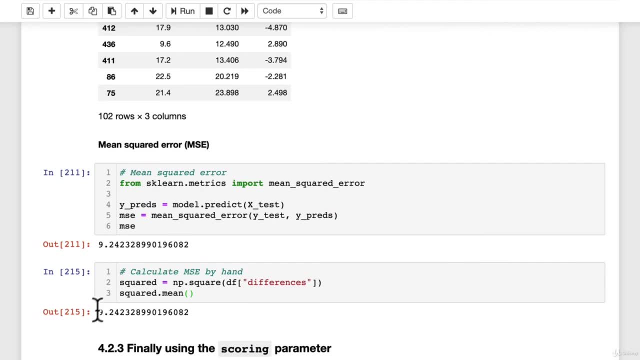 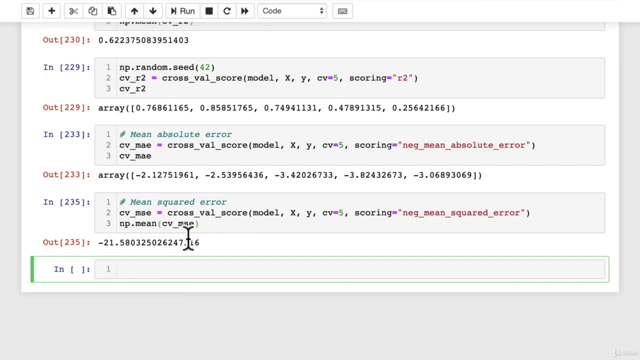 when we weren't using cross validation. right Of mean squared error is 9.24.. Hmm, So naturally, if we're looking at these evaluation metrics and we're starting to see, okay, we wanna get better metrics, you might be starting to think is like: 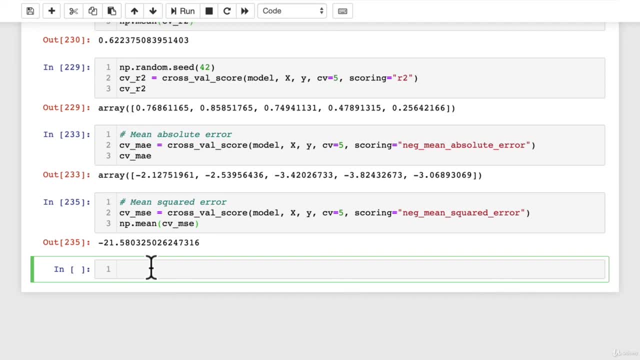 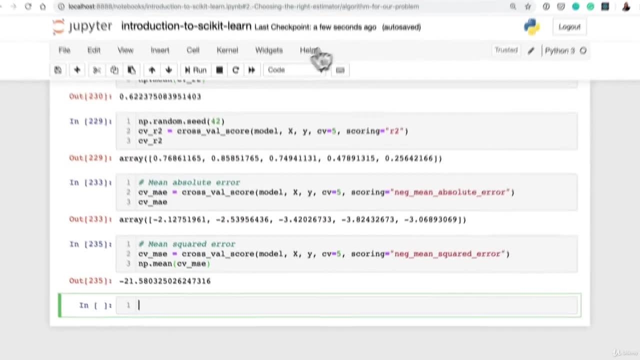 how can we start to improve these metrics, How can we make them better? And we're definitely gonna look at that. But finally, to finish the evaluation metric section off, we're gonna have a look at the third and final way of of evaluating a model, and that is using metric functions. 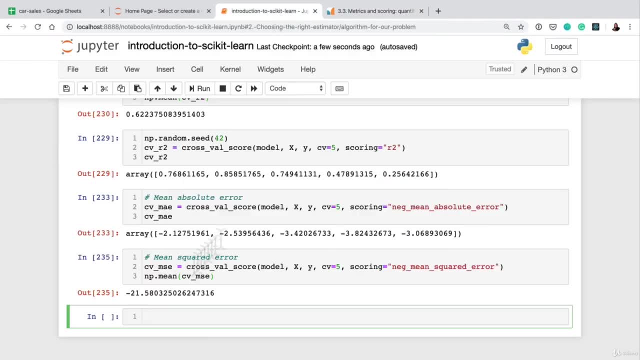 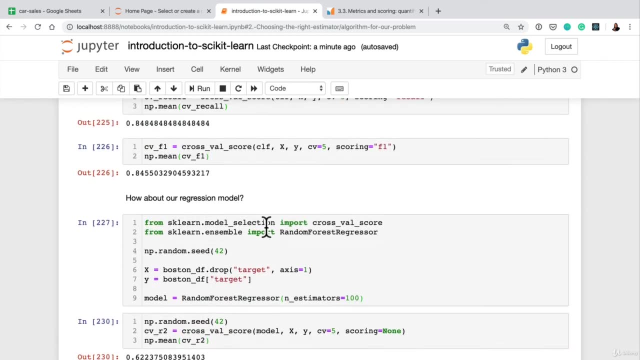 Spoiler alert. you've seen some of these in action before, Just to make sure we're evaluating our models correctly. we're gonna have a look at those, So take a little break. We covered a lot in this video. Try adjusting the scoring parameter yourself. 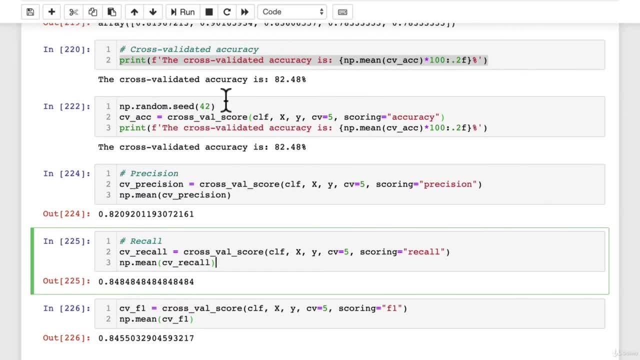 Don't forget, if you're getting different values, you might be using a different seed every time, And I'll see you in the next video. 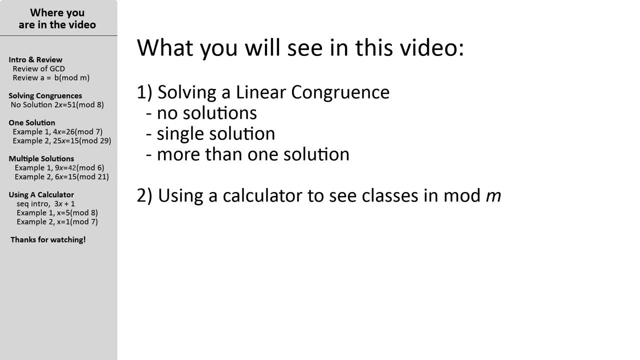 Hey there, YouTube viewer. This video will show you two things: The basic technique of solving linear congruences and how to use a Texas Instruments graphing calculator to help you generate congruence classes of modulo m. Before we dive into it, it's important. 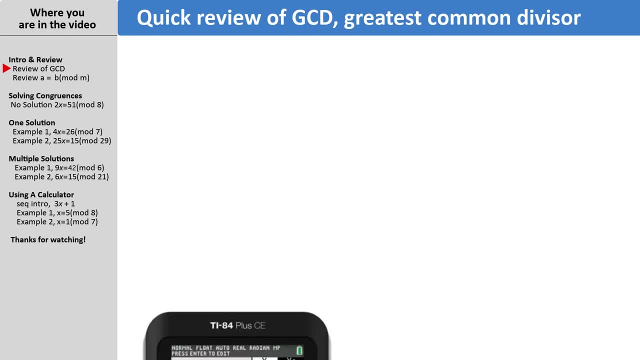 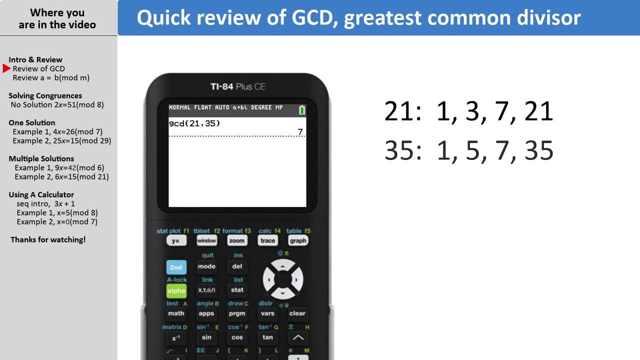 you have a solid understanding of greatest common divisor. Some calculators have built-in functionality for finding the GCD. If it's been a while since you've seen GCD, then simply find all the factors of both numbers, line them up side by side and identify the greatest. 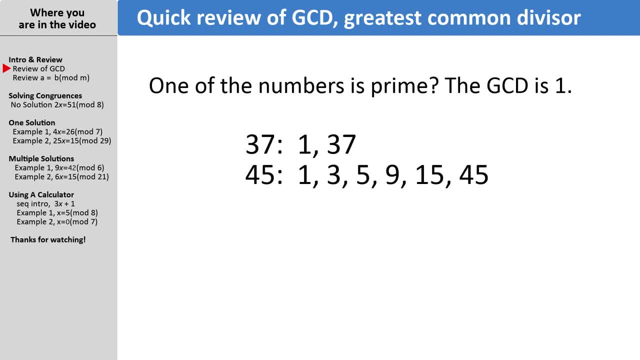 common factor like. so: If one of the two numbers happens to be prime, that's great because you can take a shortcut and simply say the GCD is 1.. Alright, the main topic, A linear congruence, has this form: a is congruent to b mod m. 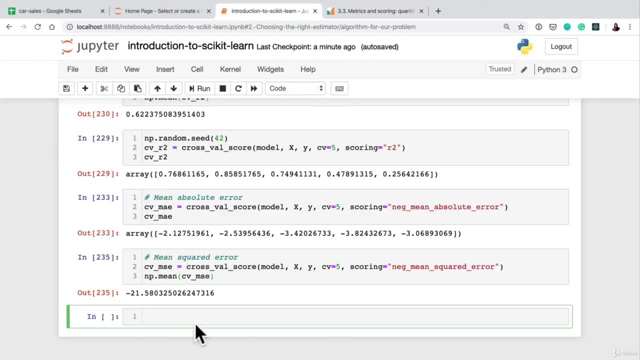 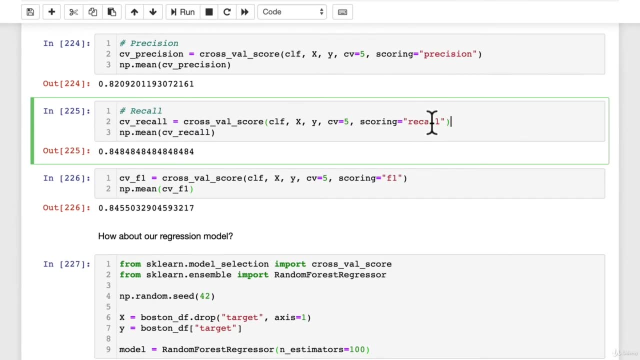 Just to make sure we're evaluating our models correctly. we're going to have a look at those, So take a little break. We covered a lot in this video. Try adjusting the scoring parameter yourself. Don't forget if you're getting different values. 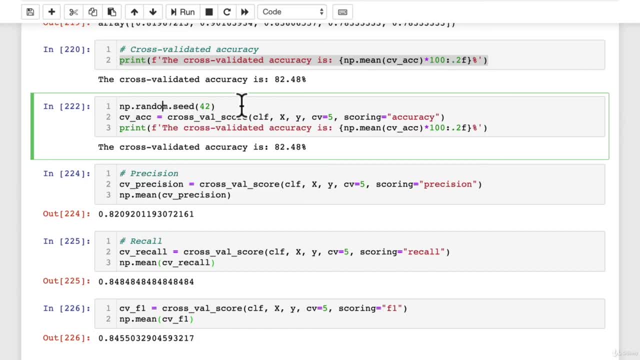 you might be using a different seed every time, And I'll see you in the next video.